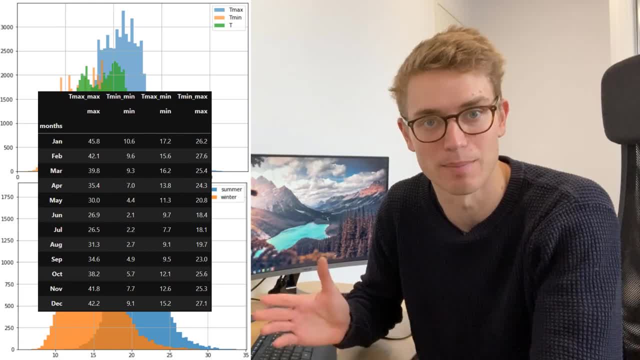 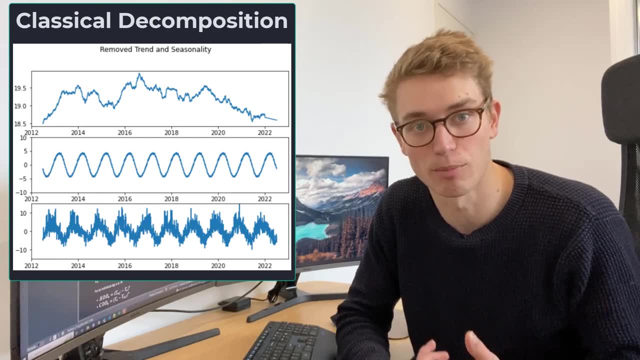 differences between weather and winter periods and maximum and minimums over given months. We're then going to use time series, classical decomposition to be able to detrend and then remove seasonality from our data set. Once we do that, we're going to use an autoregressive model, a time series model. 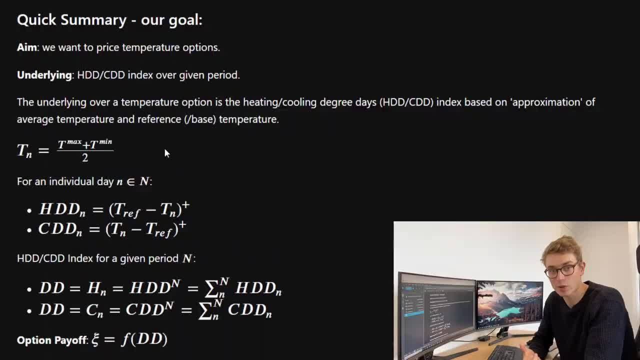 to be able to model the errors that we're left with. So just a quick summary of our goal of this series, which is actually to price temperature options. Now a quick reminder that the underlying here is heating degree days and cooling degree days index over a given period. So these HDD and 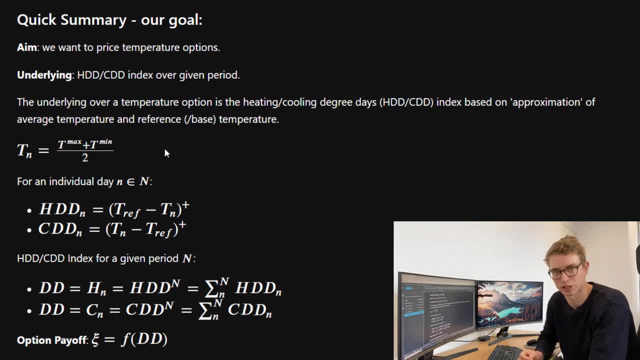 CDD indexes are based off the approximation of average temperature, which, in many places around the world, is just the average between the observed maximum and minimum temperatures throughout the day. So for an average temperature, we're going to use the average temperature index. So for an 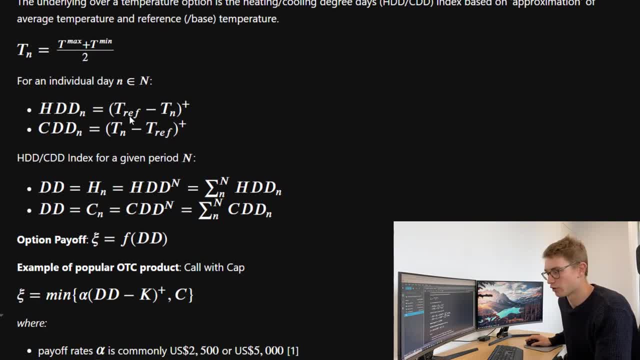 average temperature index. we're going to use the average temperature index. So for an average individual day we have an HDD of the T of the maximum of zero between the T reference temperature or base temperature minus this average temperature, And for cooling degree days it's just the. 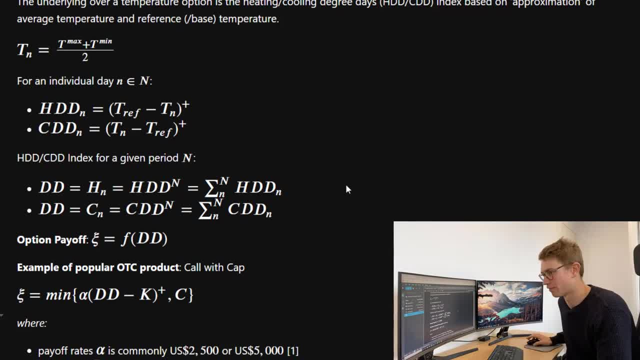 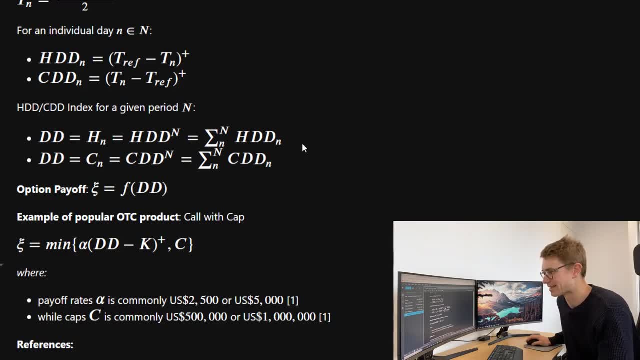 opposite. So the HDD and the CDD index for a given period in, for example, the winter period or the summer period, is just going to be the summation of all those days, HDDs, the heating degree days and the cooling degree days over that given period. Now the option, payoff- is really. 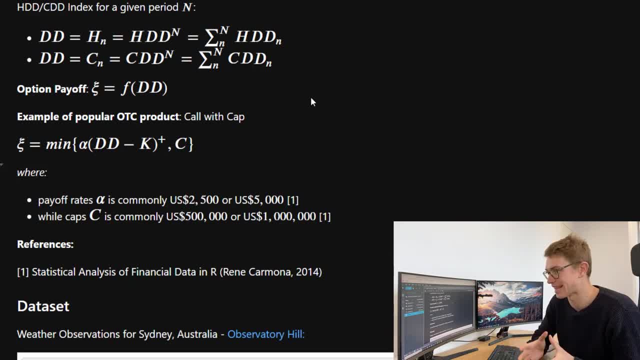 only limited by the fact that it's based on this heating degree day or cooling degree day index. But other than that, let your imagination run wild. But exemplar products that actually trade OTC are, for example, the call with a cap And this is the form where you take the minimum of a, either the 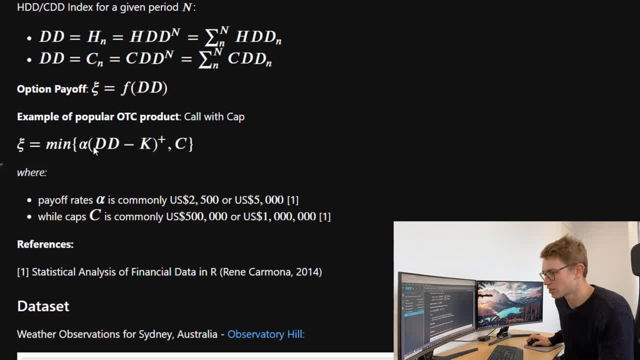 cap- commonly $500 or $1 million USD, and this average rate payoff for every heating degree day over a specific temperature. So, for example, the call with a cap and this is the form where you take the minimum of a- either the cap- commonly $500 or $1 million USD, and this average rate payoff for. every heating degree day over a specific temperature. So, for example, the call with a cap, commonly $500 or $1 million USD, and this average rate payoff for every heating degree day over a specific temperature. So, for example, the call with a cap and this average rate payoff for every. 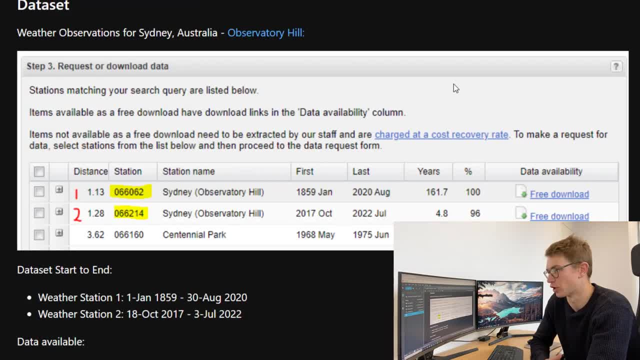 heating degree day over a specific temperature. So, for example, the call with a cap and this opposite for the put. So, with that goal in mind, let's move on to the data set that we're going to be using Here in Australia. I live in Sydney and I'm really interested in actually doing a bit. 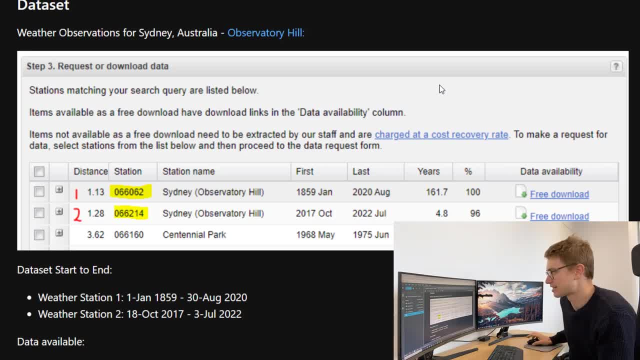 of a weather analysis of the Sydney data set. Now the data set that I'm using is from BOM, the Bureau of Meteorology here in Australia, And here we can actually get data going back to 1859, which is pretty incredible. I've had to stitch two bits of data together. It looks like they've got a. 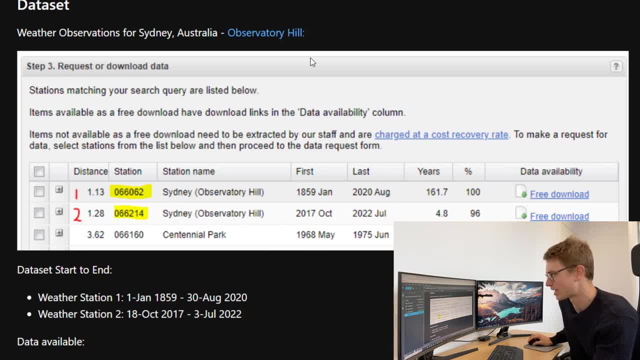 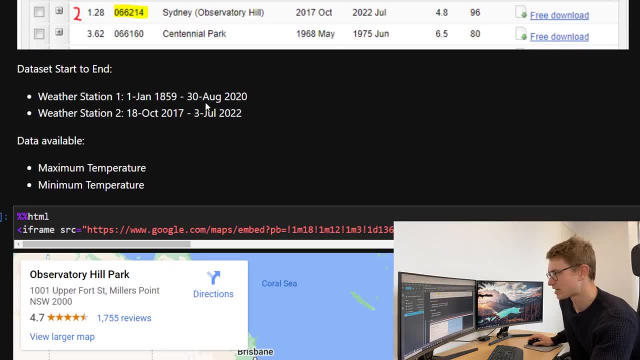 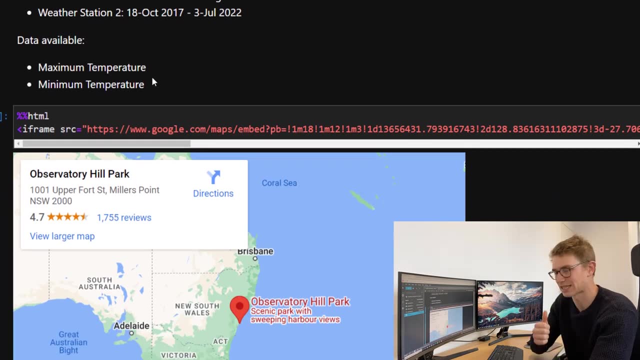 recent weather station and update at the Observatory Hill. The link is here and in the description. So with those two weather stations in mind, I've stitched that data together, downloaded it from the website and then got the CSV files- Now the data available, essentially. 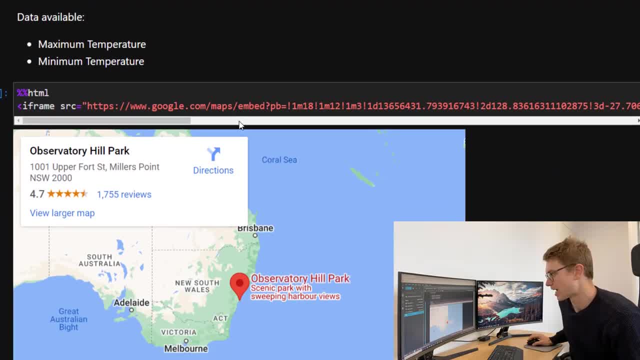 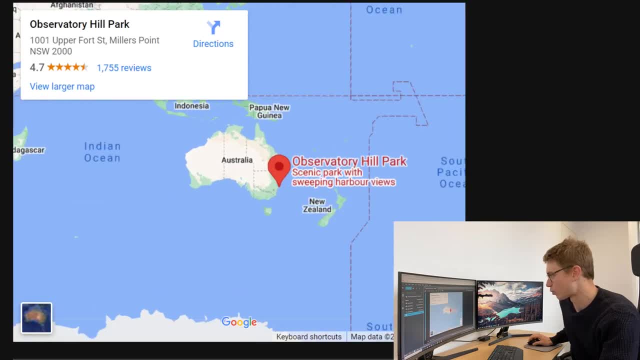 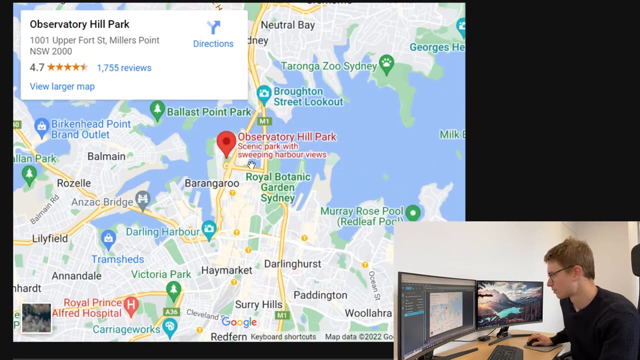 I've got maximum temperatures and minimum temperatures. Now, for those of you who don't live in Australia: Sydney is on the east coast of Australia, in New South Wales, And if we zoom in it's right near the Sydney Harbour Bridge. Observatory Hill is there, So we're going to be. 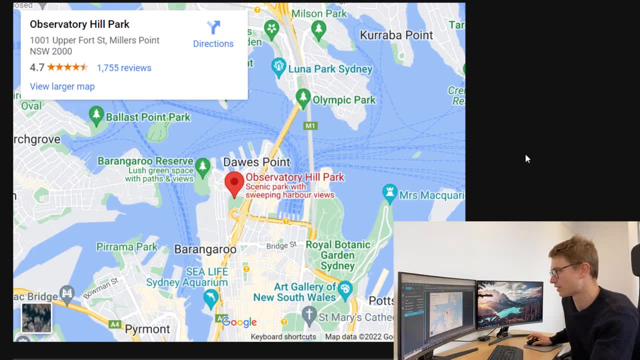 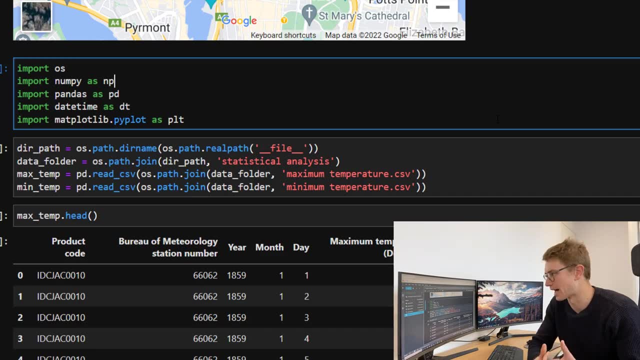 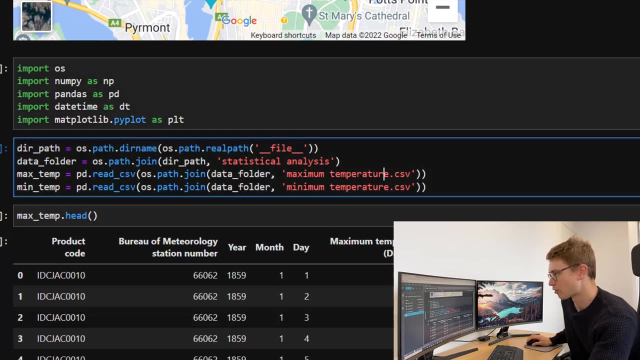 looking at these two weather stations at that location over the last- yeah, greater than 150 years. So let's import our dependencies. We've got NumPy Pandas, DateTime and Matplotlib Here I'm just going to reference where I've downloaded those maximum temperature and 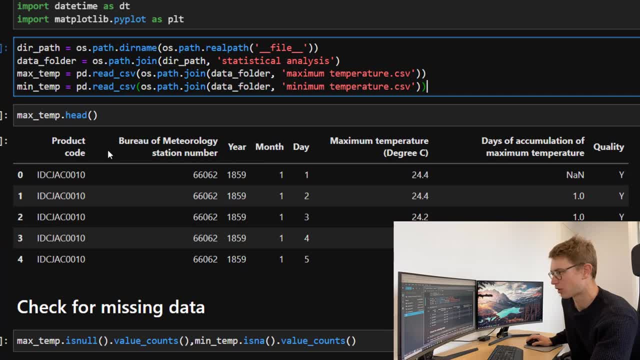 minimum temperature files And essentially here's what one of them look like. I've got product code, a BOM station number, so that weather station number. I've got years, months, days maximum temperature. This is the column that I'm interested in, And then the 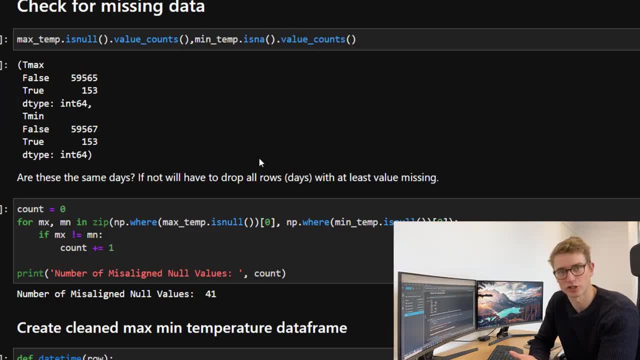 quality of the data. Now, because this data set is so large and it goes back so many years, it's good to check for missing data. So if I have missing data for one- the max temperature or the minimum temperature- then I'm not going to be able to compute my average temperature. 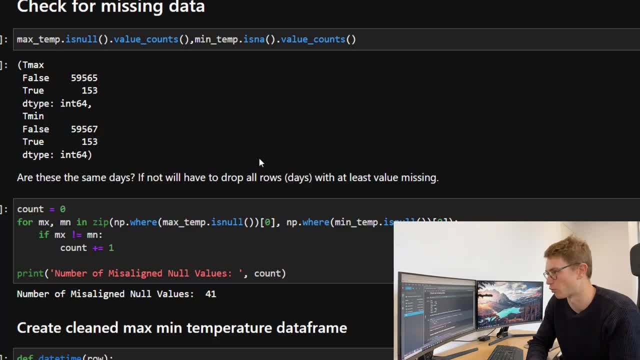 within that specific day. So it would have to remove that row completely. so i'm checking for nulls here and here we've got true, 153 from the max and 153 for the min, but, like i just said, these might not be occurring on the same day which. 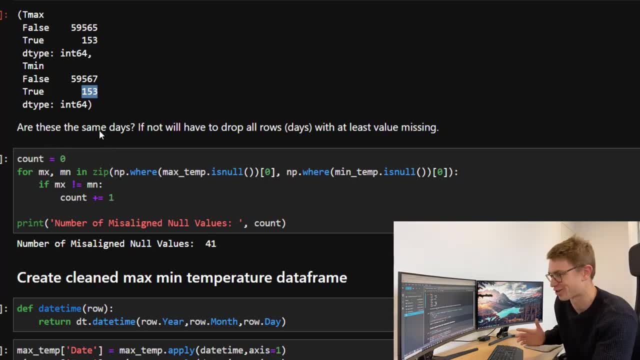 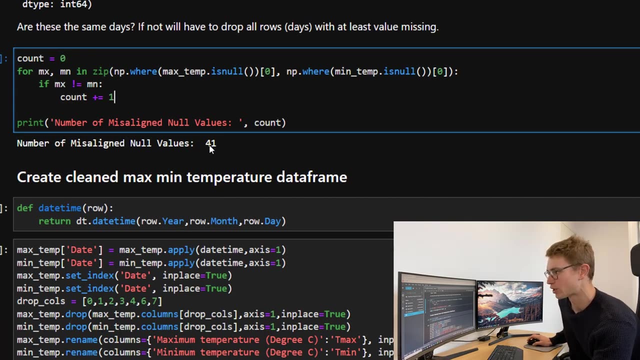 is annoying, so i asked myself the question: are these occurring on the same day, and what we can do. we can just zip these two data frames where this is null and i want to return back if these are occurring at the same point and we in fact find out that 41 of the 153 missing data points 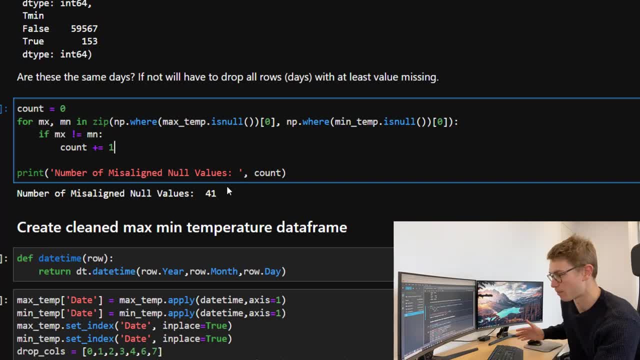 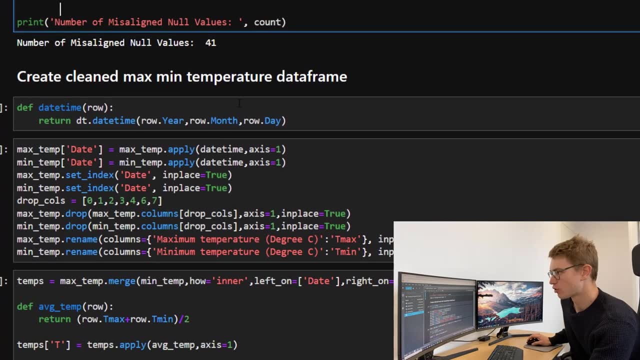 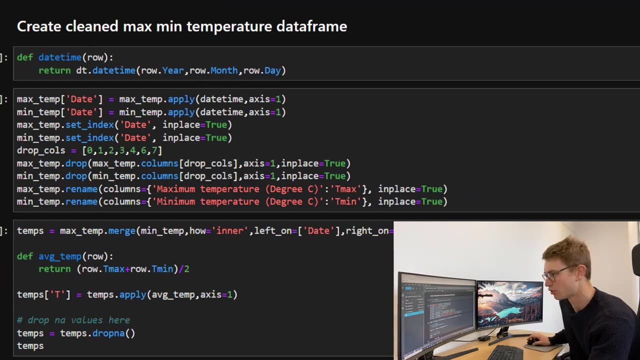 do not occur on the same day, so that's annoying. i'm just going to have to remove all those rows after i make the transformation of that average temperature. so here i've got a bit of code that i've created and cleaned up the max and mean temperature data. fame, remember. i'm only interested. 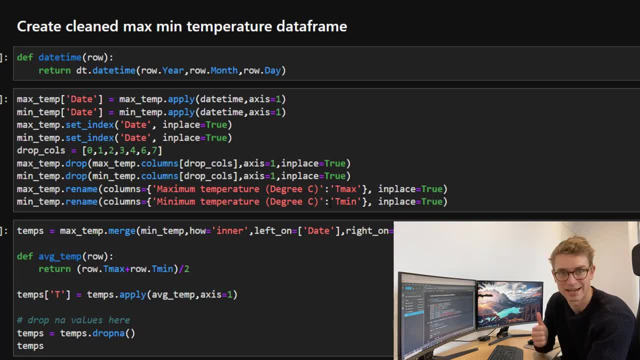 in the maximum temperature column and the minimum temperature column and then the actual date. so i change everything to date times, i apply that change to the data frames, set the indexes date and drop all the other columns, and then what i'm going to do is rename the maximum temperature. 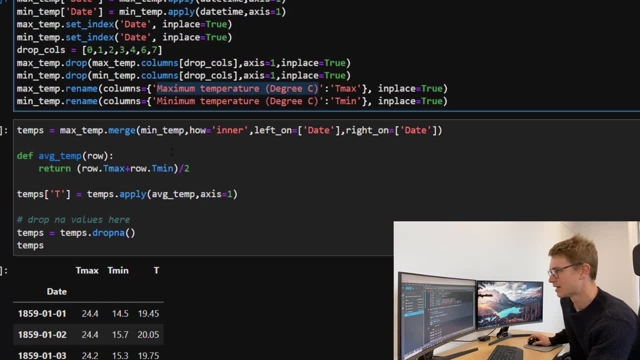 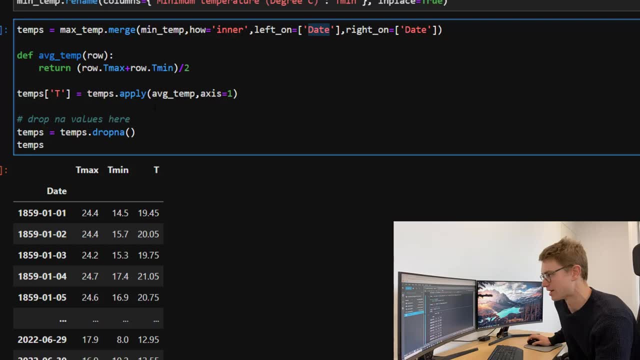 column and minimum temperature columns to t max and t min, then i can join the two data frames and i join them as an inner on left and right on both the date indexes. once i've done that, i can use a function- average temp- and that's just going to take the row and the indexes and i'm going to 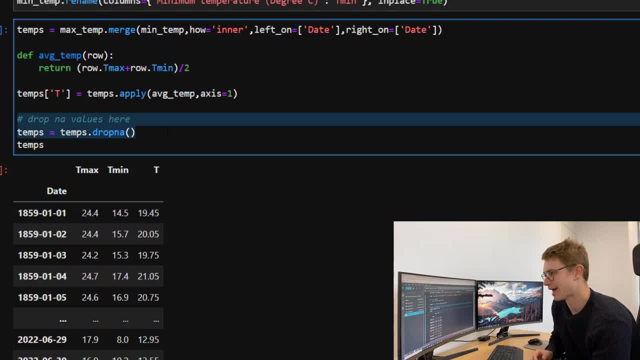 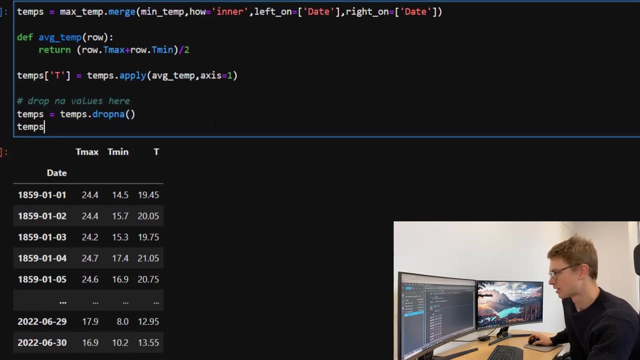 go t max and t min and divide it by two, and then, once i've done that, now i'm going to drop all rows on na values and remember i have to do that because if i didn't have one particular temperature for a minimum max, i am not going to have a correct average temperature. so once we've 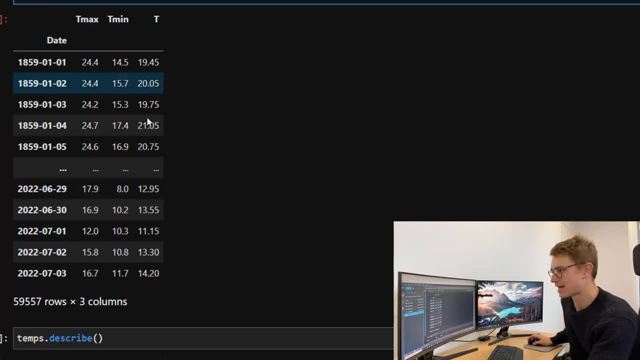 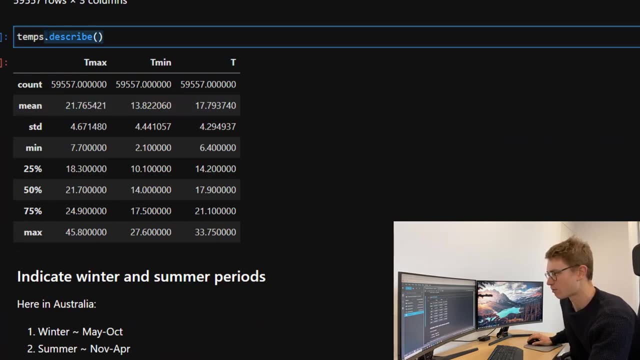 done that. our data frame looks like this and i've got dates: t max, t min and temperature. to look at some general statistics about this, we can look at the describe function from pandas. this can give us a count on all the rows of data. so you know nearly 60 000 rows daily. information of 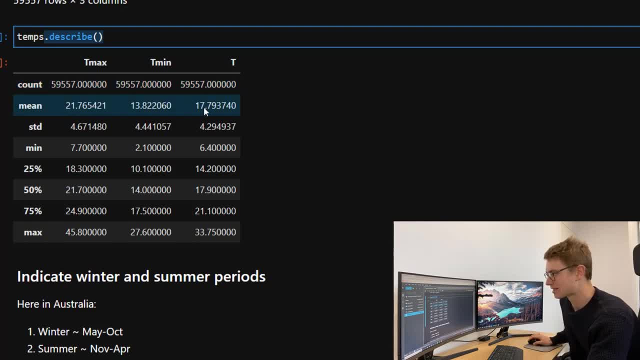 temperature, which is crazy. we can look at the means of the t max, t min, and then average temperature, standard deviation and then some of the percentiles and the min and max. now, this min and max is pretty cool, but this is over the entire period. what happens if we want to? 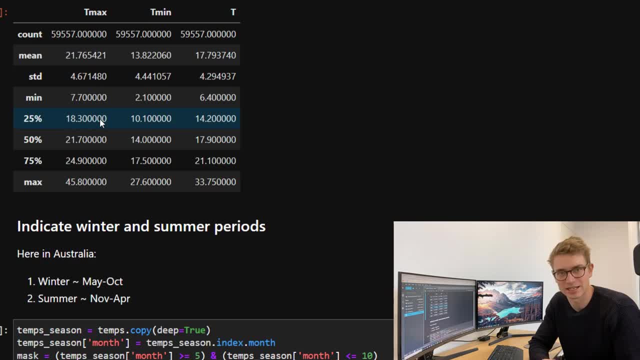 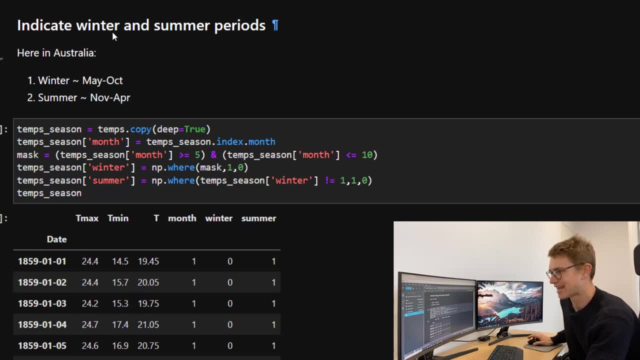 look down at particular months or seasons to get a bit better idea of what the max and mins have actually been. so first thing i'm going to do, i'm going to indicate the winter and summer period. so here in australia i've got winter being the period from may to october, and 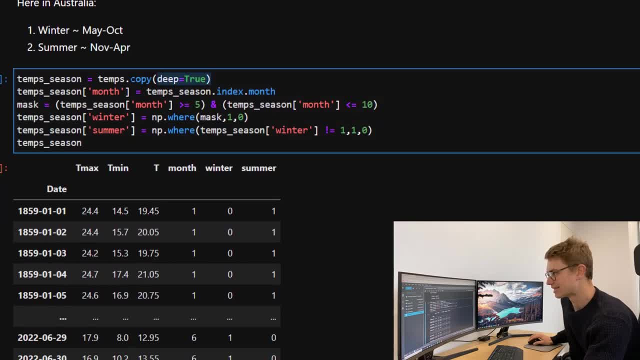 then summer, from november to april. so i'm going to do a deep copy on my temperatures data frame and then i'm going to label a season as the month which i'm just taking, the index month. i'm then making a mask, which is the specific temperature. 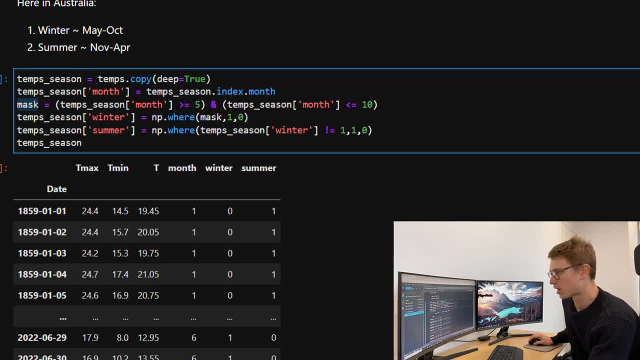 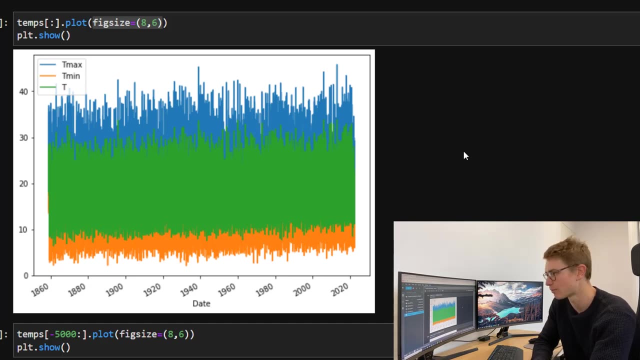 season of the month, months for winter, and then i'm applying a that mask to my filter, making the indicator equal to one if it's winter, and then i just do the reverse for summer. now visualizing the data, here's just a time series plot of our three indicators: t max, t min and temperature over the uh plus 150 years. 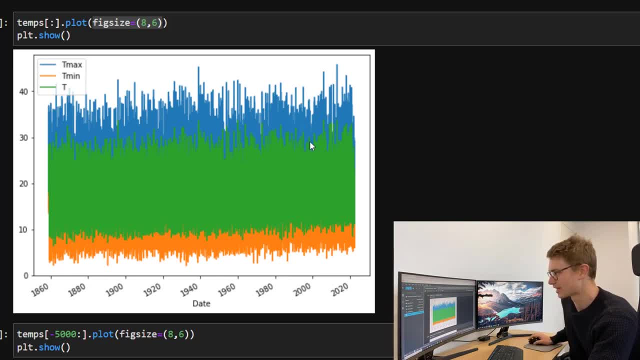 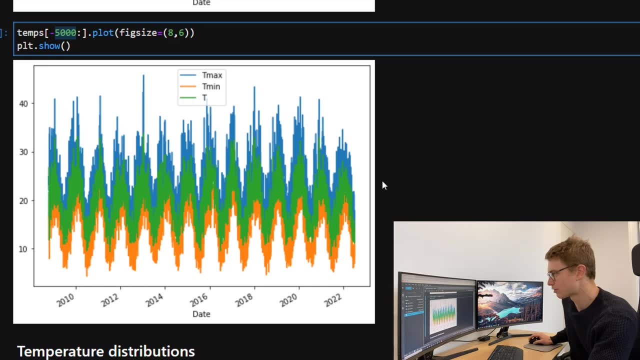 i mean. so it's not very useful. i can't really see any oscillations, so let's zoom in a little bit. i'll just look at the last five thousand um, or you know know, 12 year period, and here what we've got is we can see in blue our t max, t min is below and we 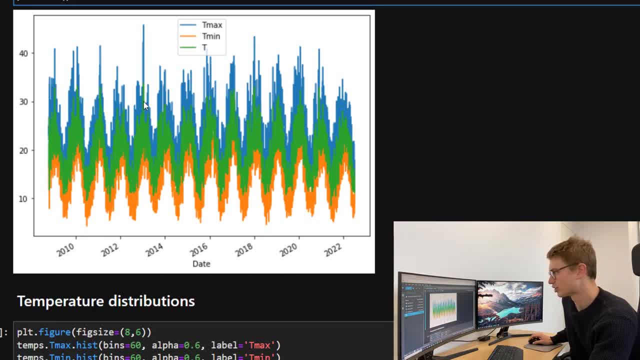 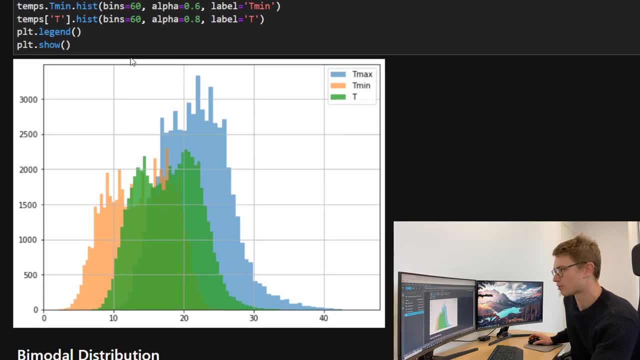 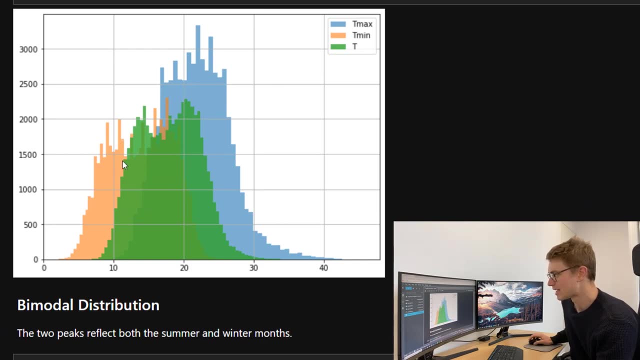 can see these huge cycles and variation in the data. so let's take a better look at the temperature distributions. so for this i'm going to be looking at histogram plots. so here our histogram plot of the t max is in blue, t min is in this orange color, and then we've got a bimodal. 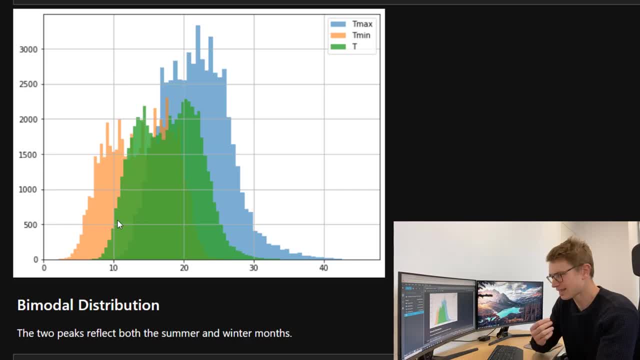 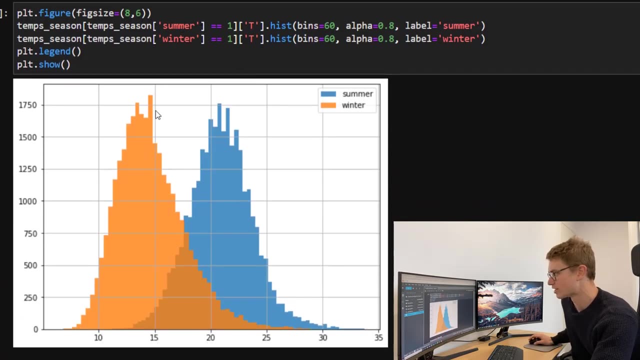 distribution here for our average temperature, and what we can actually see is this bimodal distribution with two means- the means are actually centered and reflect the peaks of both the summer and winter months- and to show that we can then use our indicators for our summer and winter months. 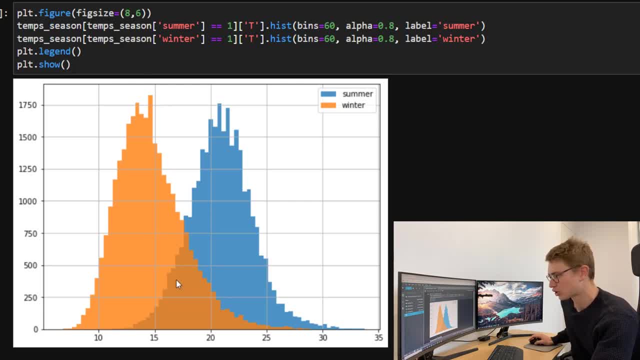 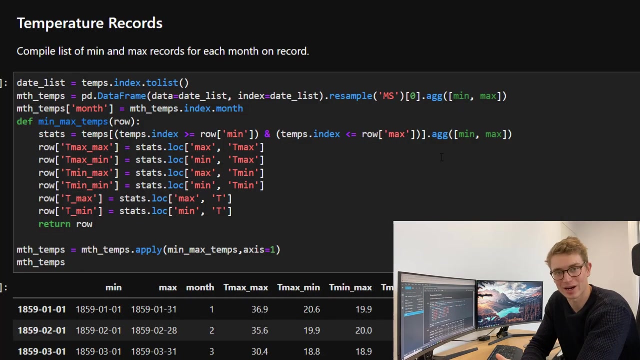 separate this distribution into two histograms and show that over time. here is my slightly negatively skewed distribution for the winter months and then somewhat more normally looking distribution for the summer months. so interesting here to see that the temperature distribution in the southern hemisphere here is negatively skewed. so now i'm quite interested in seeing the temperature records that have actually materialized. 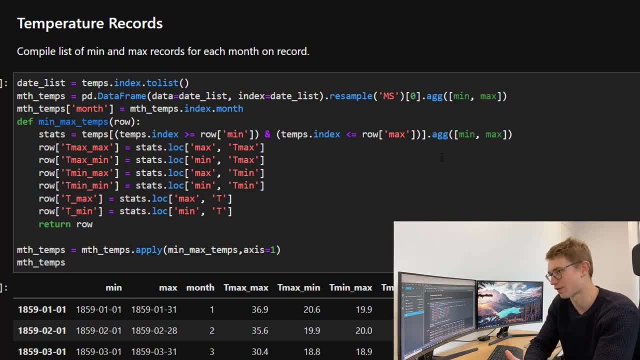 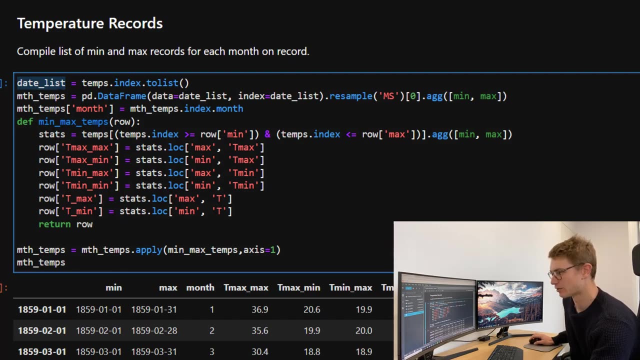 for particular months, and this is just satisfying a curiosity, but you could do it on whatever season you want. so let's first compile a list of min and max records for each month on record. so the way i'm doing this, i'm compiling a date list for my time series data frame. i then need to resample on. 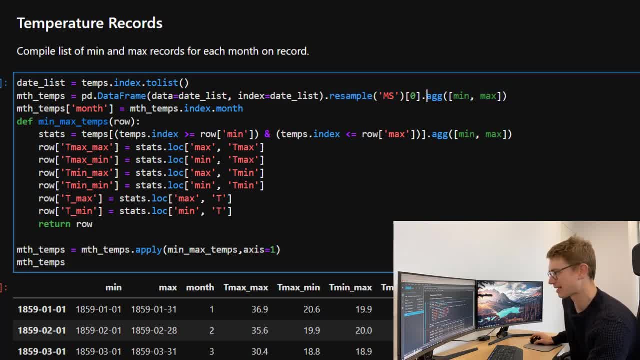 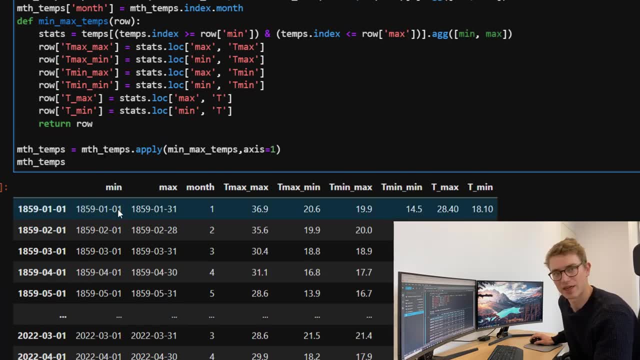 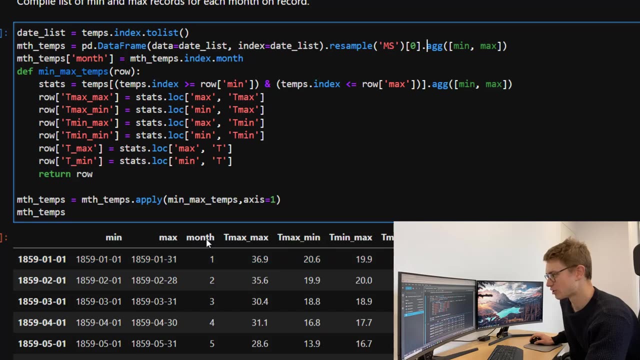 the monthly starts and then i'm going to aggregate the min and max. now, once i've done that, i can aggregate a data frame for each particular starting month, with the min of that month and then the max of that month. i can then create a index which is going to be the month that that's on. so 1, 3 to 12. 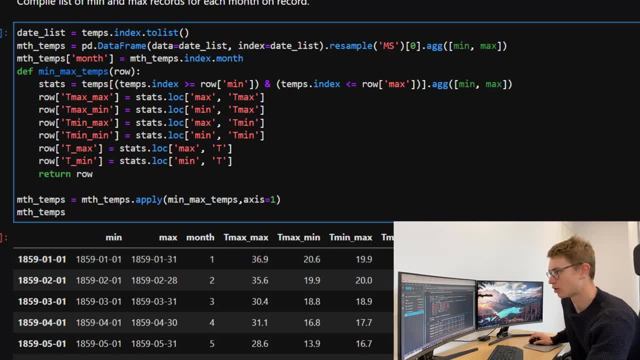 from January to December and we can aggregate that on that later. then we can subsection our original data frame temps each time based on what month we are in. and here we're just going to take the maximum temperature and we're going to take the max of the maximum temperature observed and the min of the maximum. 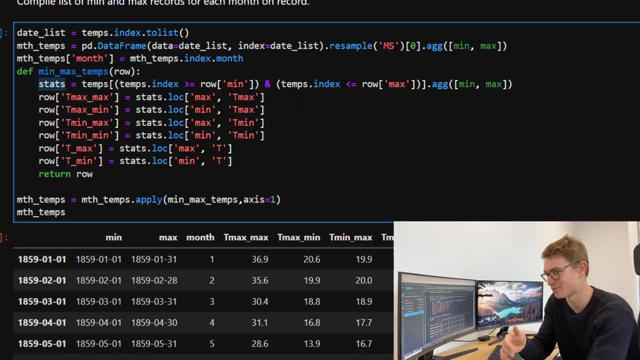 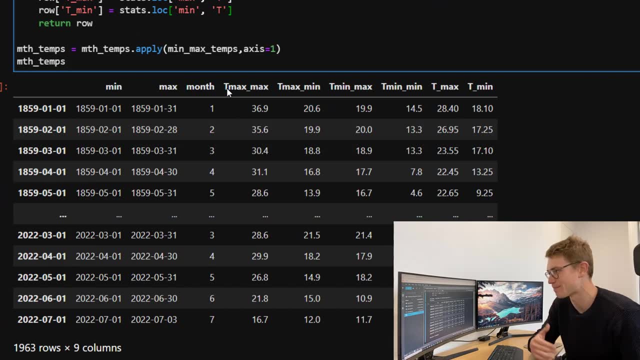 temperature observed and then the max and min of the temperature min observed. we're also going to do this for our average temperature, so I know that's a bit confusing, but we- yeah, essentially we're looking at the max and min that is observed within a particular month of the team acts, the tea min and the. 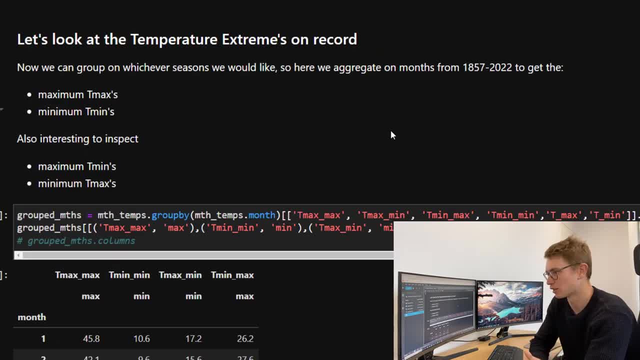 temperature profile. so let's take a better look at the temperatures extremes that exist on record, now that we can group these seasons however we like. so we're going to look at the maximum T maxes and the minimum T min, because obviously this is the most interesting. we also 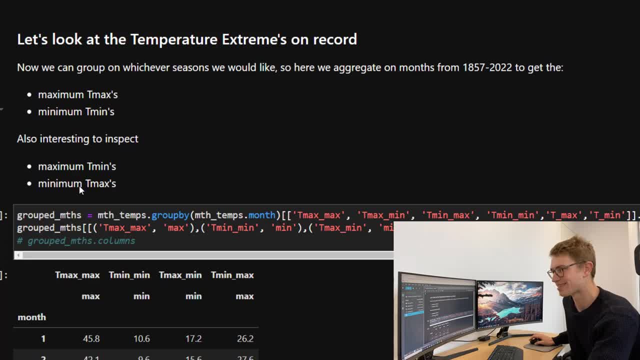 interesting. we're also interested in that because when we look up, we get more interested in looking at the maximum T-mins that were observed and the minimum T-maxes. So here this is like the maximum temperature that you might observe for a particular month. 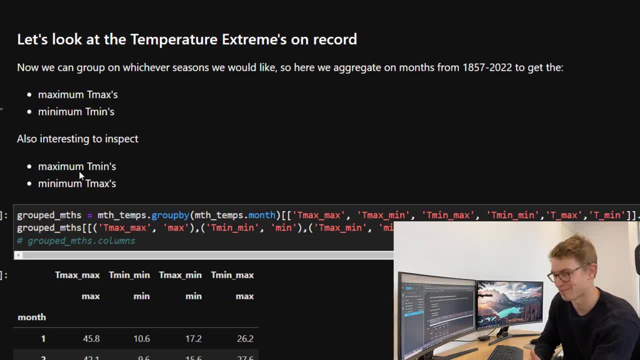 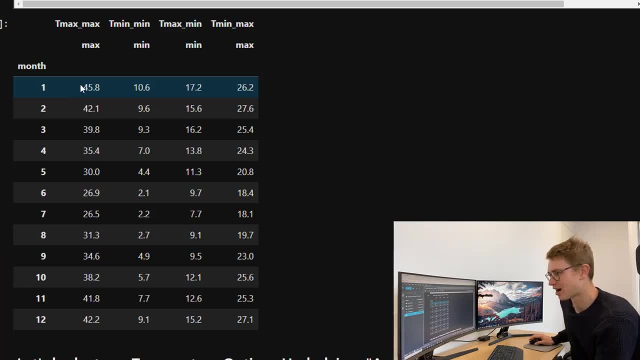 You might be interested in seeing the maximum T-min in the winter months. Once we apply that group by, we end up with a data frame like this, And interesting to see that the highest temperature on record that I can see for the Sydney Observatory is 45.8.. 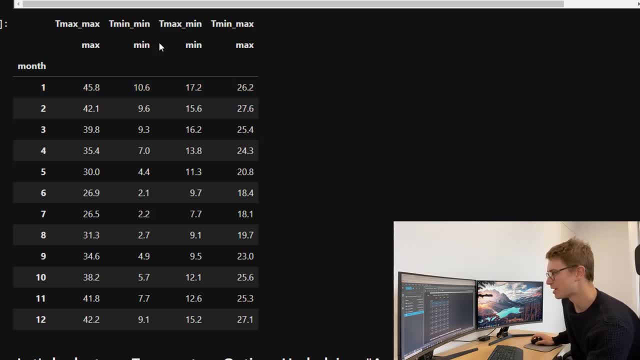 And obviously you can go back through the data and look up where that occurred. Now the minimum temperature that I can observe- that's happened on record at the Sydney Observatory- is actually in the June period here at 2.1.. But it's important to know that the min temperature, the maximum of the min temperatures that have 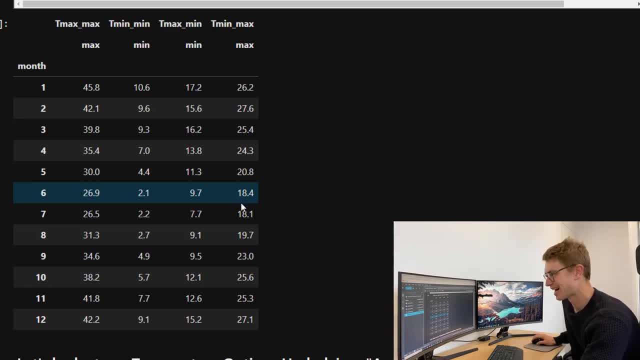 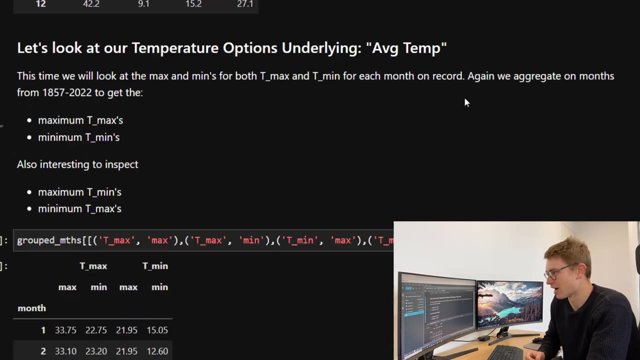 ever been observed during that height of the winter period, for June is actually 18.4.. So it's interesting to see these swings in the extreme temperatures Over that well, 170 year period. nearly Now we're going to look at our underlying, which is that average temperature indicator. 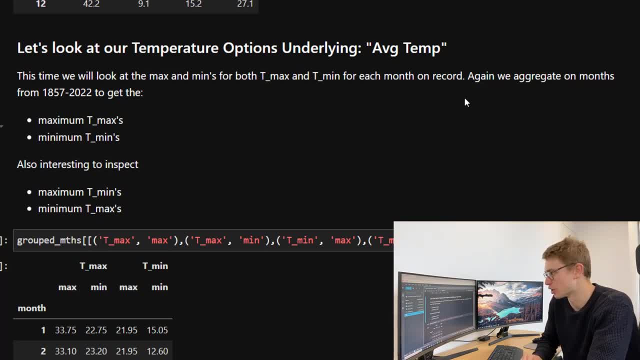 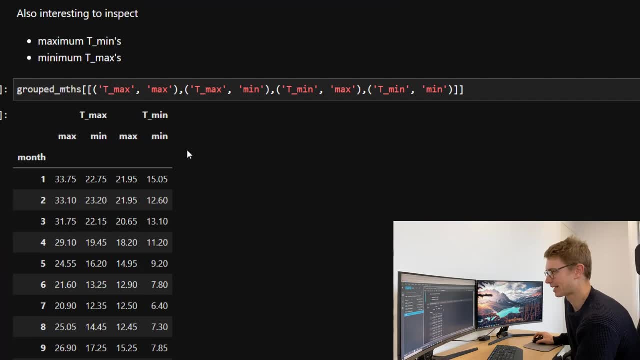 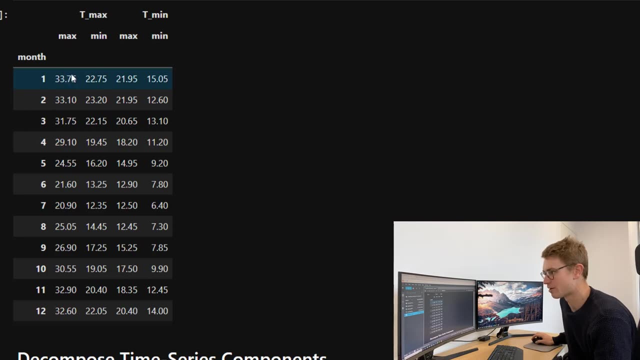 So we're going to look at the maximum and minimum observed for each individual month. We're also going to look at the maximum T-mins and the minimum T-maxes. So this is our actual underlying data, that average T, and we're interested in the maximum. 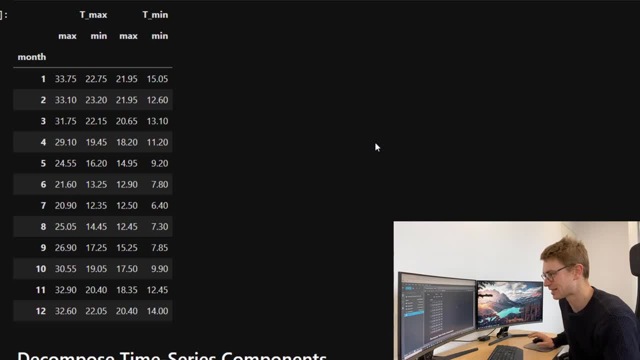 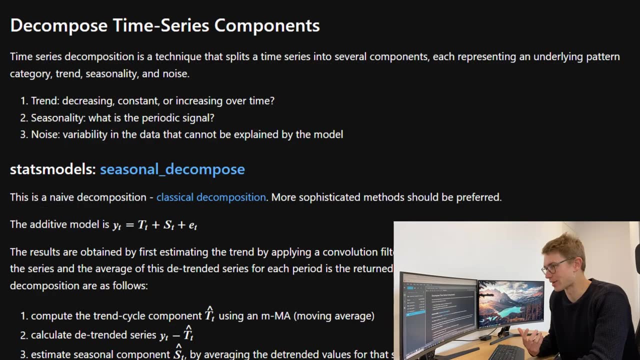 and minimums observed. So that's how you can compile it. So different seasons. Now that we've looked at the statistics, let's jump into how to decompose this using time series. So now we're actually going to model and do time series decomposition. 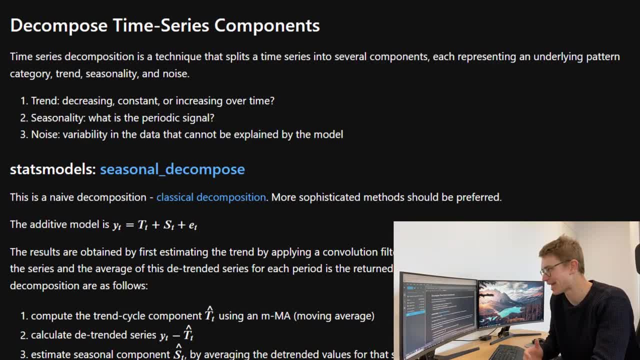 So this is a technique that splits the time series into several components, each representing an underlying pattern in the data. So here we're going to talk about trend, seasonality and noise. Now usually there's a third component called cycles, but this is actually going to be taken. 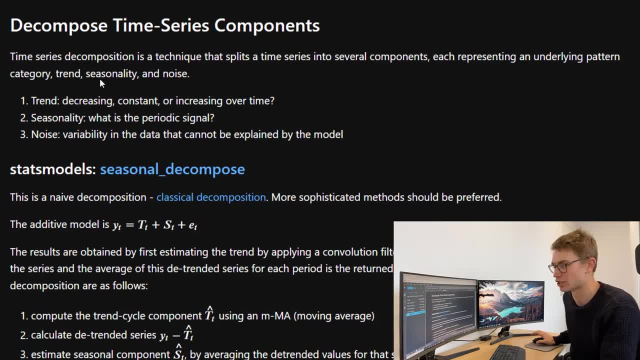 up in classical decomposition into the trend component. So really It's a trend and cycle component. So is the trend decreasing, constant or increasing over time? What is the periodic signal for the seasonality and the noise? So the variability in the data that cannot be explained by the model. 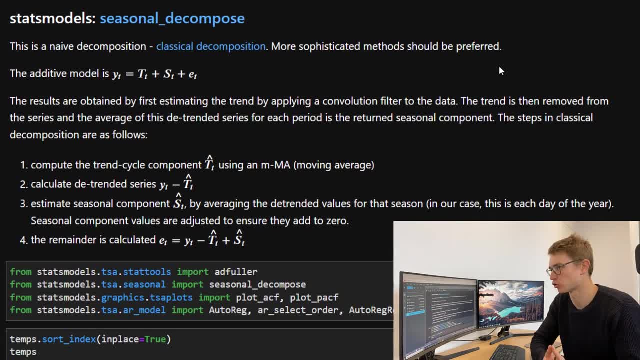 This is really the remainder, So by stats models, seasonal decomposition: this is a naive decomposition used in Python and it uses classical decomposition. So what is classical decomposition? Well, essentially, the additive model is of this form. here Again we have our time series varying with t, with our trend component, our seasonal. 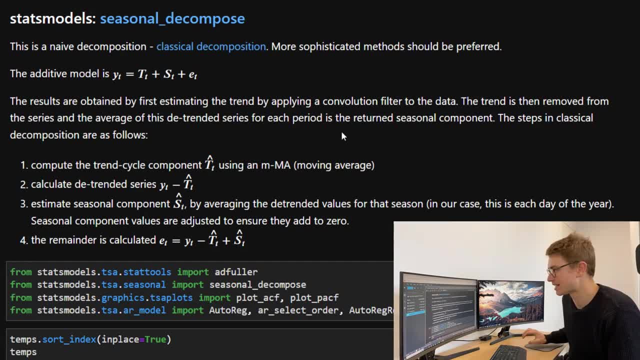 component and then our error term. So the algorithm is using a convolution filter on the data. The trend is removed and then the average of this detrended series is used for each period to actually return the seasonal component. The steps for classical decomposition are as follows. 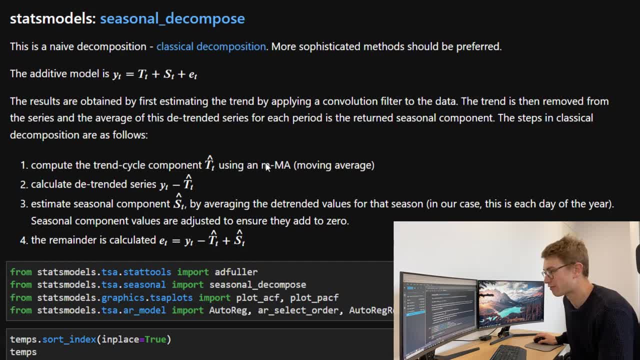 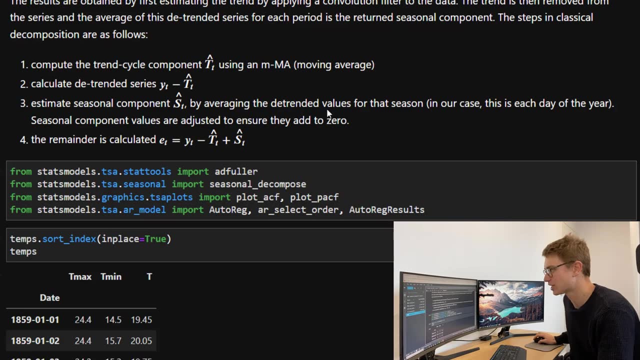 So here for the trend cycle component over a given period, m, So the period we're going to define. we can get a moving average term, Then we can take this away from our original time series to get the detrended series. The estimated seasonal components is then calculated by averaging the detrended values. 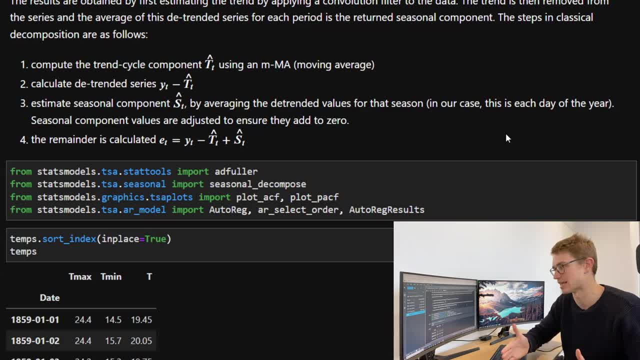 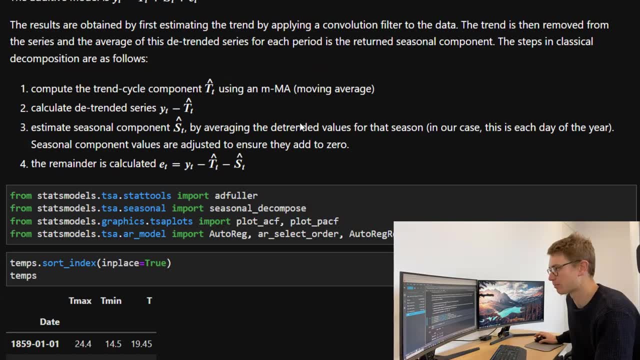 for that season, And in our case this is going to be every day within the year. So the seasonal component values are then adjusted to assure they add to zero, And then this remainder and error term is just calculated by subtracting the trend and 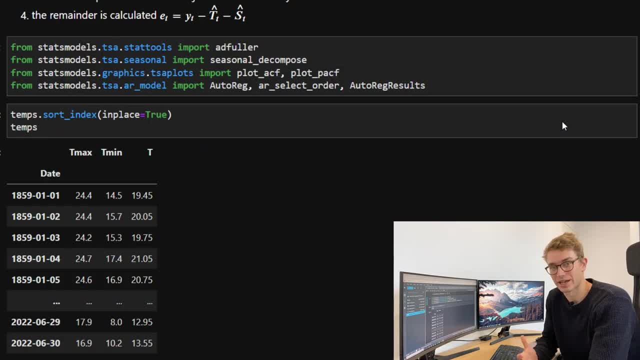 the seasonality from our original data set. So we'll talk about the distribution. We'll talk about the disadvantages of using classical decomposition in a minute, But for now let's import our dependencies. So, from stats models let's import the AD fuller test, which is the unit stationary. 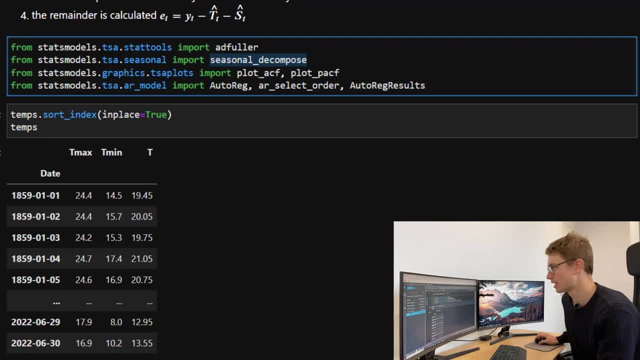 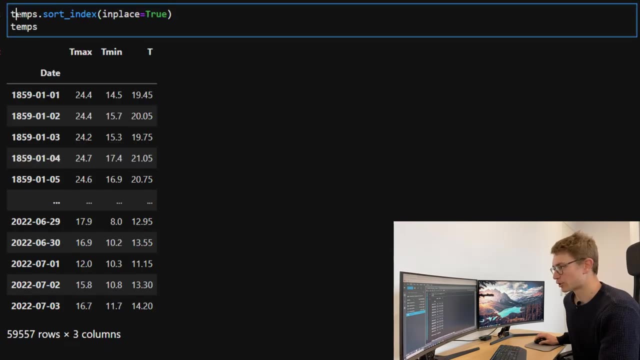 test. We'll import seasonal decompose. We'll use the plot ACF and plot PACF for partial autocorrelation functions and autocorrelation functions, Autoreg, AR, select order and then autoreg results. Again, our temperature frame It's going to be. I'm just going to sort on the index which is our date. 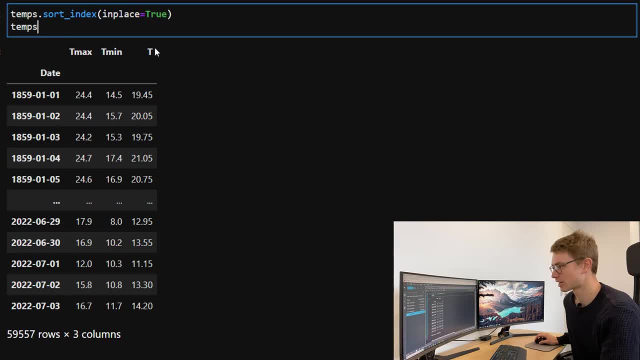 And here's what it looks like. We've got Tmax, Tmin and temperature. Remember, we're only interested in temperature. And then our date time series goes from January 1859 all the way through to today. Now let's just take a brief look at our data set. 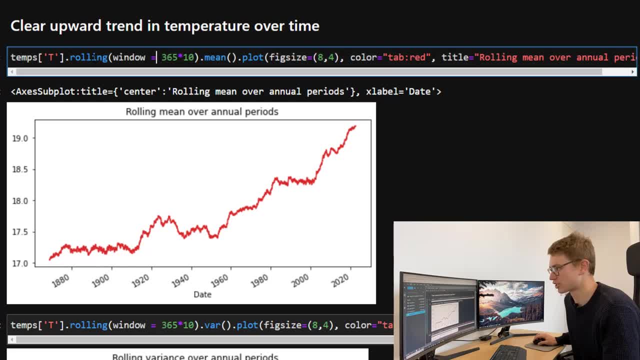 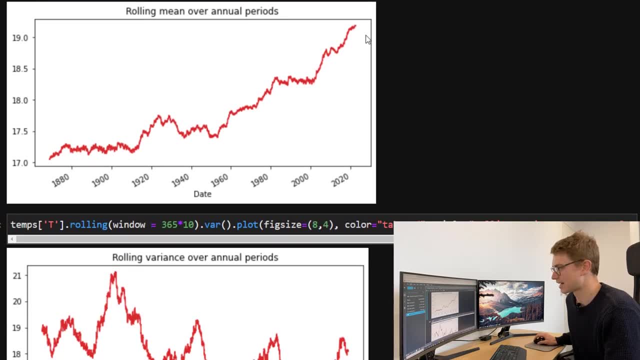 Here we have a clear upward trend in temperature over time. I've just taken a rolling window of 10 years, got the mean and plotting that over time And here you can see that I've tripped over time and I've also taken the variance over that time window as well. 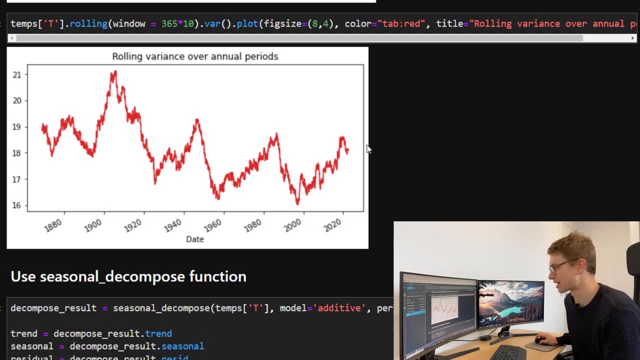 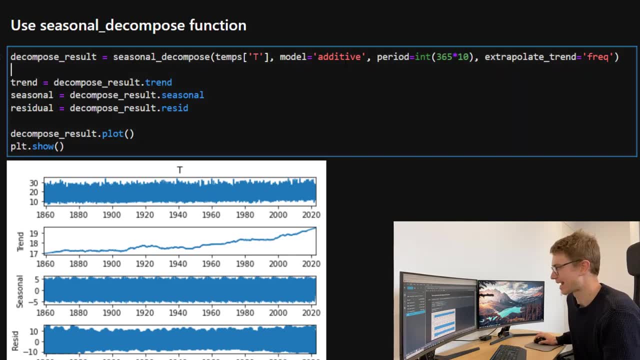 And you can see that variance has definitely changed over that time period. So, with that in mind, let's use our seasonal decompose function. So here we're going to use that additive model that we spoke about before. We're going to pass in our time series temperature of just T, that average temperature indicator. 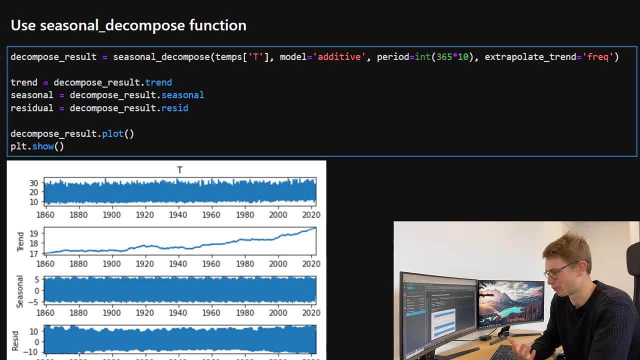 Now, because we have such a long time series- We've 15 to 16 decades- I'm going to choose a moving average term period here of 10 years. Now, this is kind of crucial for getting a bit of a smooth trend function. 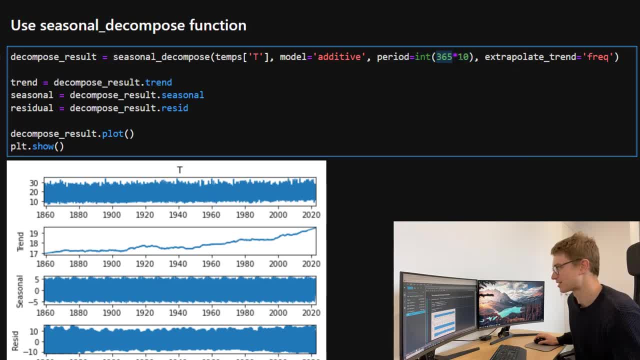 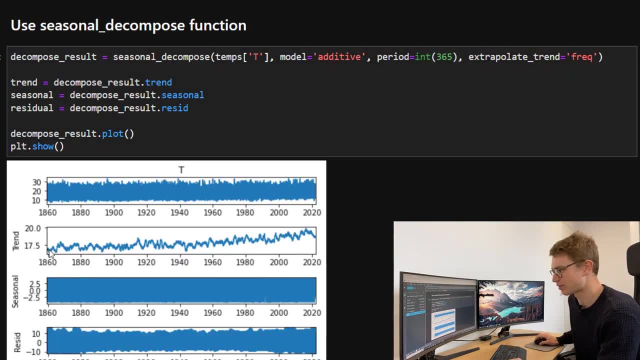 But obviously, if you want to discretize a little bit more, you can change that to 365.. And I'll just show you actually what that looks like. So if we use 365, you can see that the trend series gets a lot of variability within that. 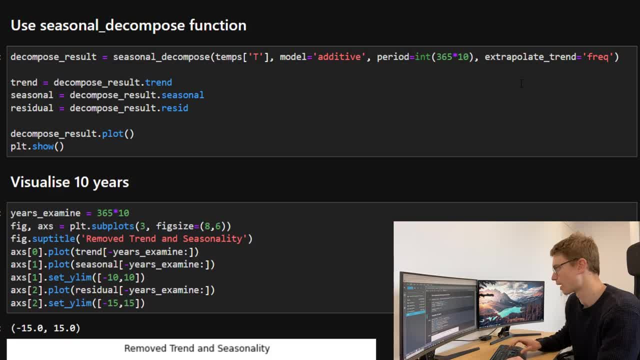 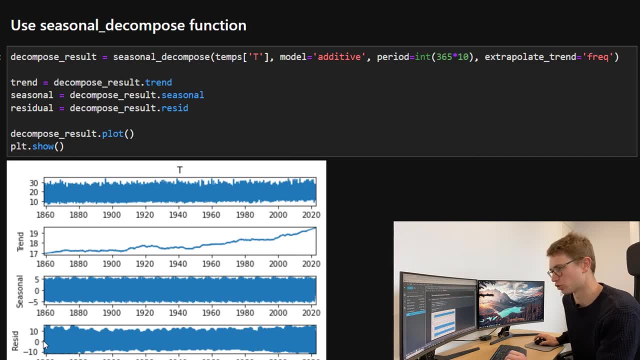 moving average over a one year period, Whereas we're kind of smoothing that out over a 10 year period, And then more of the variation ends up in our residuals and our seasonal components. We've then taken the decomposed results and then we can break it down to a trend, a seasonal 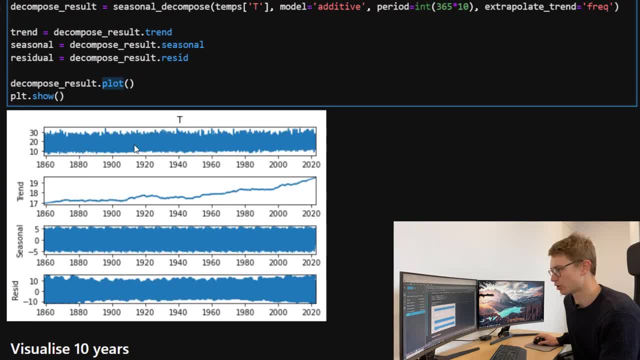 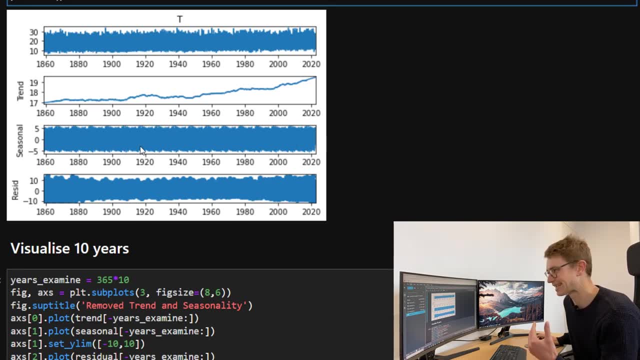 and our residual. Now, that's just the composeplot that we're visualizing there. but let's, but because everything's so jammed up and there's so many seasonal patterns to actually visualize that properly. Let's look over a 10 year period. 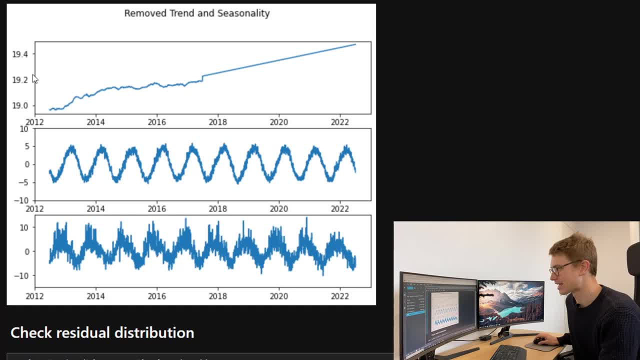 So here I'm just looking at the trend at the top, our seasonality and then our residual component. So the first thing that you're going to notice is the fact that there is this ugly straight line at the end of our data set, And the reason that's there is because we've taken a 10 year moving average. 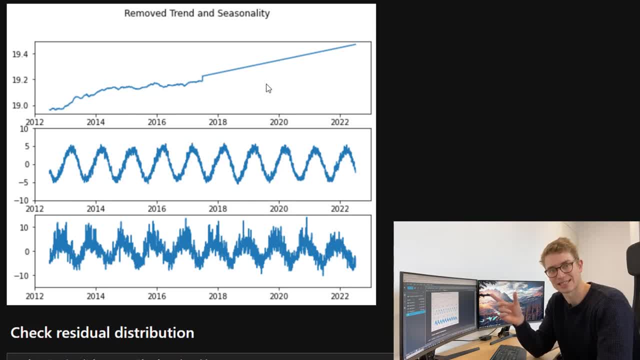 Now this is a two sided moving average, which means it's taken five years at the end of the time series and five years at the start of the time series. So it's a moving average term that's actually calculated over those periods. So what you can do is you can set it equal to the frequency and, yeah, essentially it's. 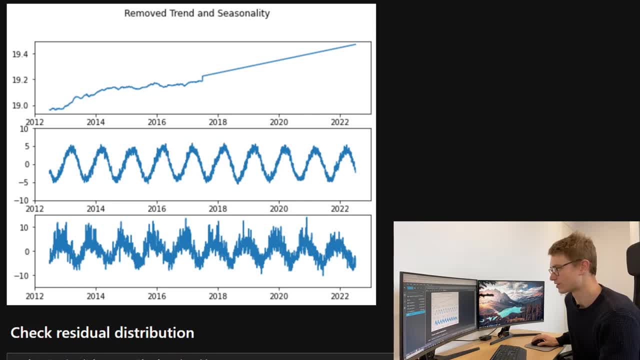 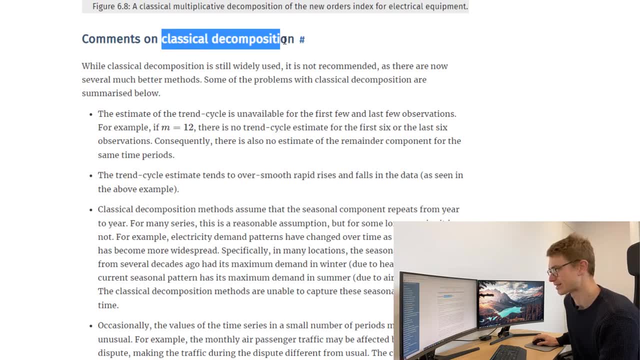 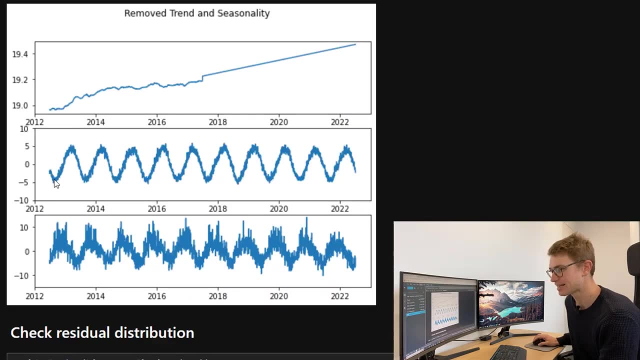 just a extrapolation, Um, and that's what we've done, but that is actually one of the downsides that's actually noted in the documentation on classical decomposition that I've given you in the link there. One of the other biggest downsides is the fact that you'll be able to see here our 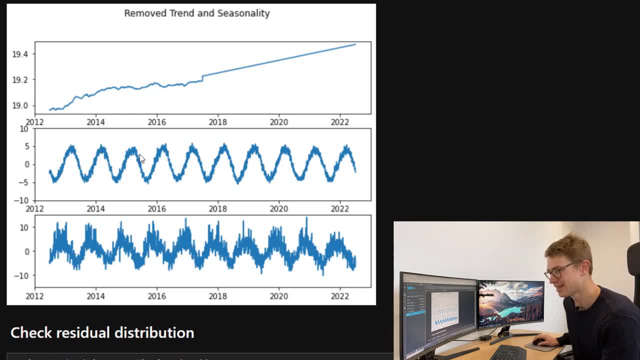 seasonality component has captured a good five degree swing. That's actually a good five degree swing. That's actually a good five degree swing. That's actually a good five degree swing. It's occurring every year, but you'll see here that there's kind of some really strong. 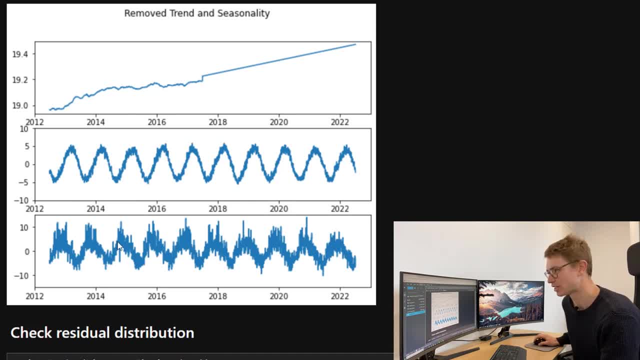 what I would call auto correlation in our residual components, and we'll see that soon. but this looks like you could almost decompose that further into a seasonal component. Now the issue here is that classical decomposition function, uh, looks over a specified amount of time and with that particular function that we're using there, it's always a one. 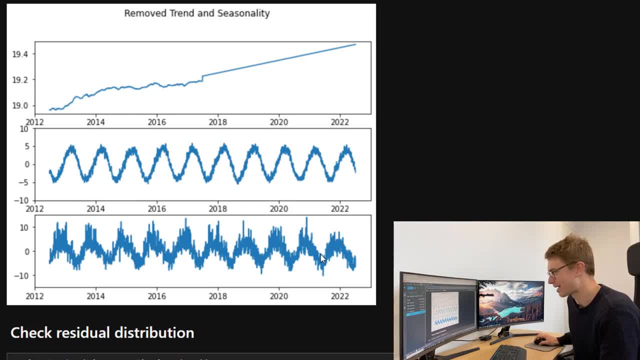 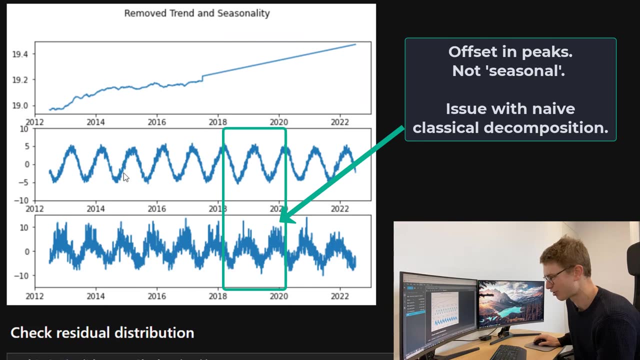 year period. Now, that's kind of annoying because perhaps we have some peculiarities um within our temperature series. That means that we've actually got um some other period or an offset, uh, to our yearly seasonal function, which it looks like here our peaks are kind of occurring. maybe you 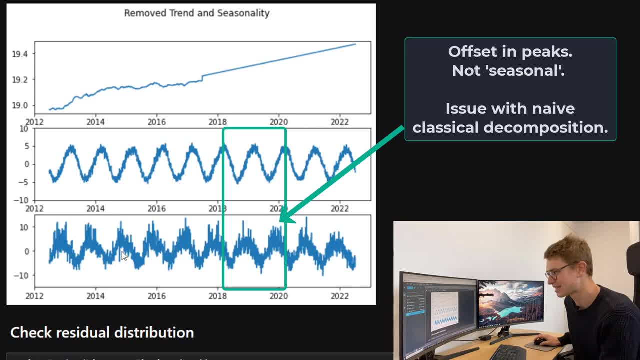 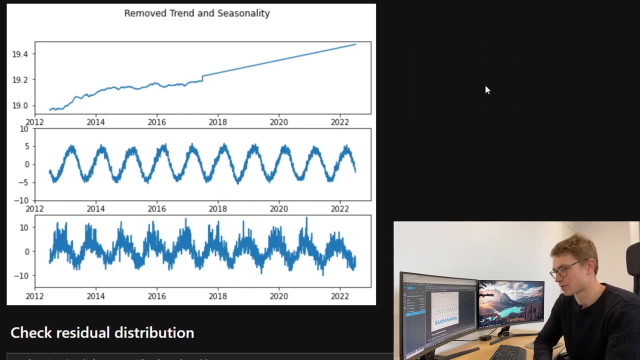 know 90 days or half a year um beforehand in our residuals. So, unfortunately, classical decomposition isn't really picking this up now, despite its limitations. we've got another method, So this is a technology that we're going to be looking at later. 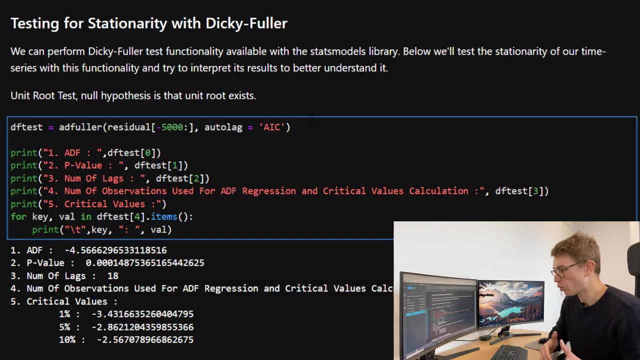 So we're going to roll on with classical decomposition. So before we do any time series um decomposition on our residuals now, we need to confirm that this residual time series is actually in fact stationary. Before we do any uh, AR or AMA models, let's perform the Dickey Fuller test. 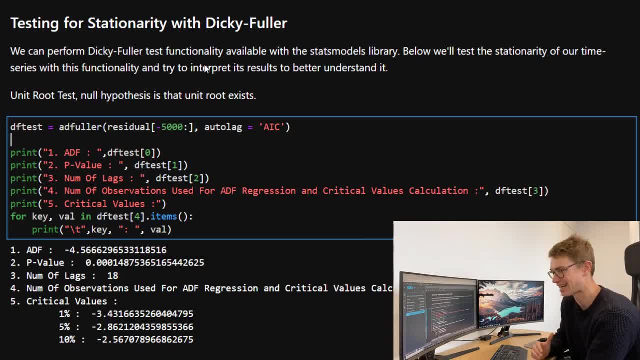 And essentially this is just a unit route test where the null hypothesis is that a unit route exists, AKA random walk. So essentially this is just a unit route test where the null hypothesis is that a unit route exists, AKA random walk. So essentially this is just a unit route test. 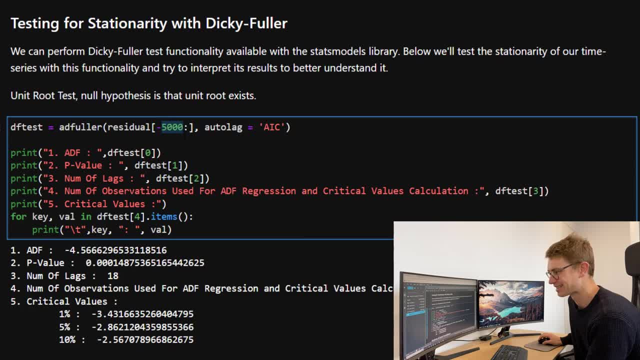 And essentially this is just a unit route test where the null hypothesis is that a unit route exists, AKA random walk. So essentially, here, what we're going to do is test the last 5,000 data points, um, and see, uh, what the results are and whether it's statistically significant or whether. 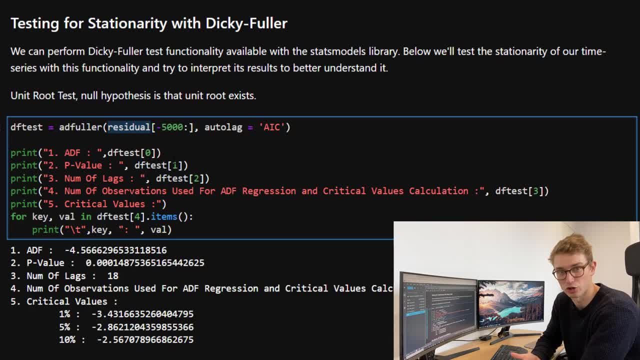 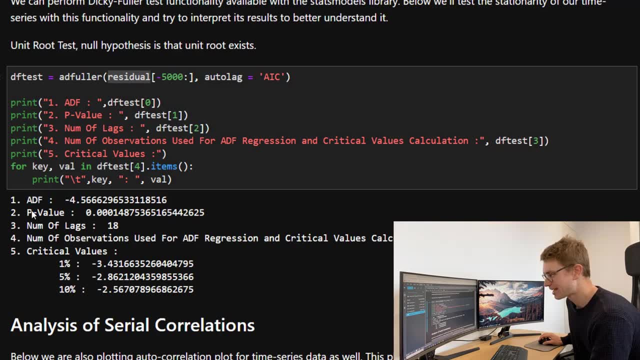 we have enough information to determine um whether a unit route exists or not. Now we've got our um ADF statistic back and that's yielding a p-value of 0.00015.. And that means that we've got enough statistical evidence to reject the null hypothesis. we've 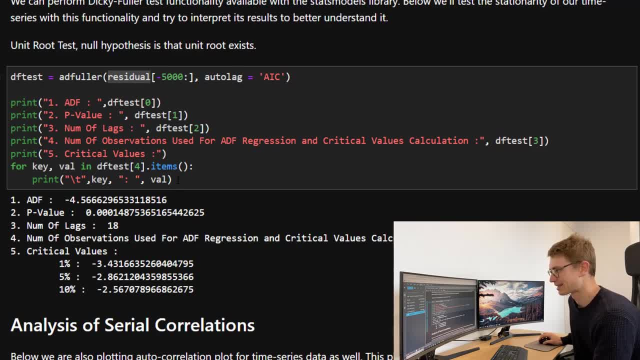 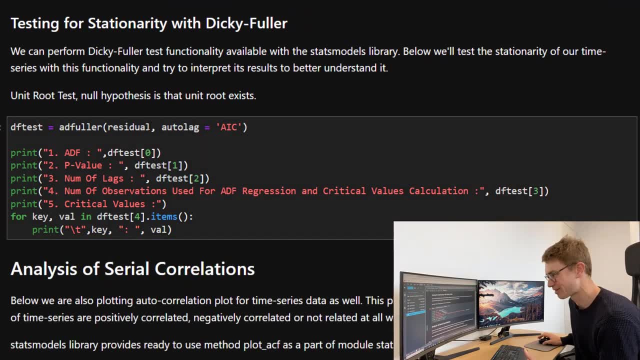 that the unit root exists. that doesn't mean that it doesn't exist. it just means that, given how data set, these are the results we've got. if you include all the data set- because we have 60,000 data points using the ADF methodology, it gets. 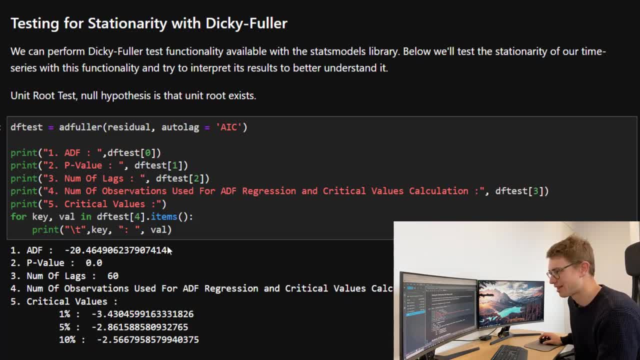 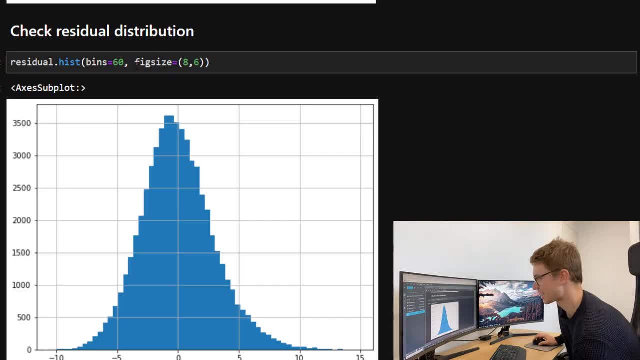 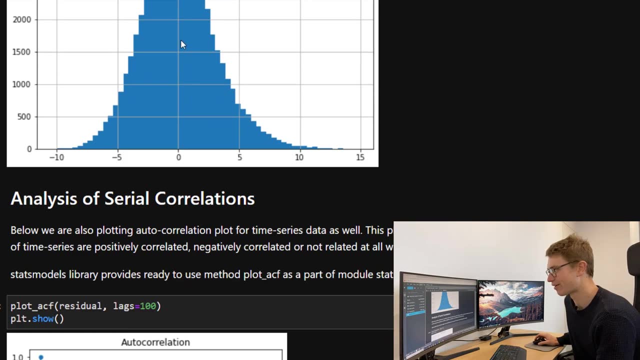 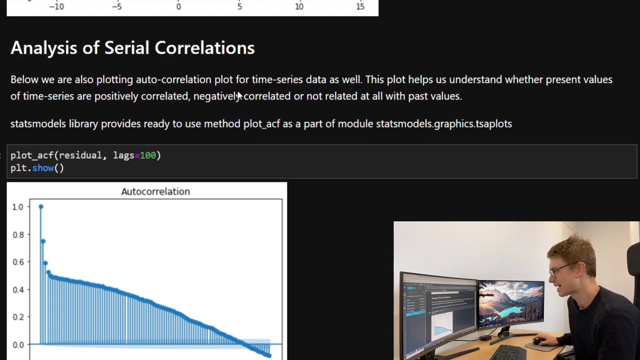 extremely likely, according to the test, that there is no unit root existing here. their residual distribution: here I've got a histogram and essentially it looks really normally distributed. however, we know that there is serious autocorrelation. so yeah, the analysis of serial color correlation or autocorrelation is just the correlation that occurs in the errors in the 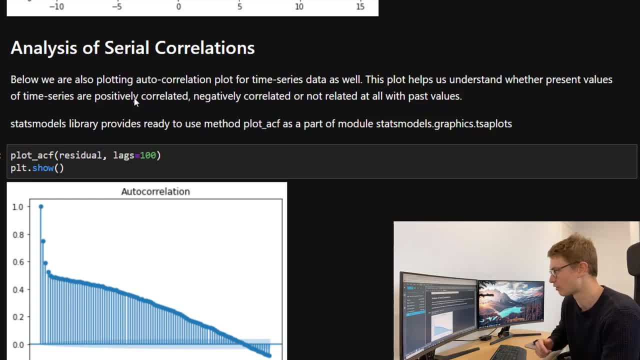 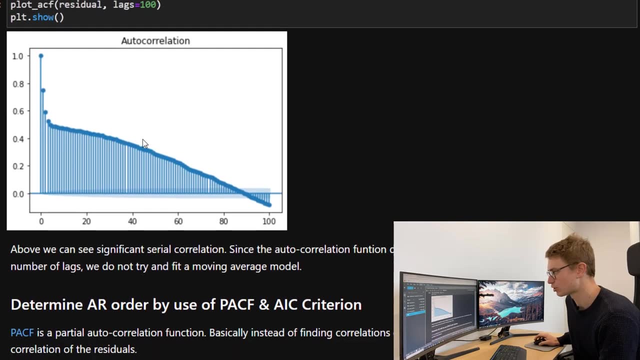 residuals from one time point on itself. so what is the correlation between a time point in the errors now compared to the last moment in time, compared to the last day, and so on? so we're observing massive autocorrelation, positive autocorrelation all the way up. 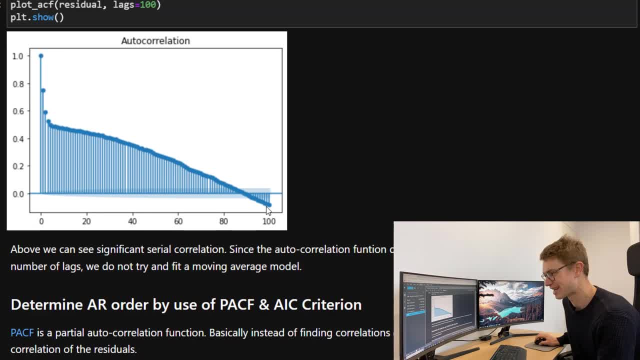 until really 90 days and then after that it just turns a negative. so exactly what this plot showing is that we have huge seasonal relationships in our residual terms over time. now, obviously there's significant serial correlation here, and since the autocorrelation function does not seem to vanish after a number of 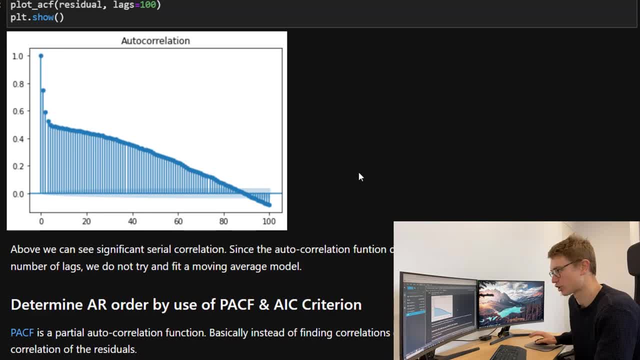 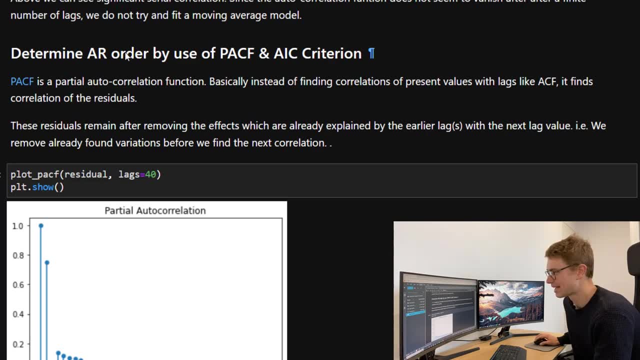 lags and we are not going to change the correlation between the errors and the percent of errors we see in the results. and the fact is that we are not going to try and fit a moving average term. instead, we're going to try and determine the number of the order, of the order of the regressive model, and we're going to do 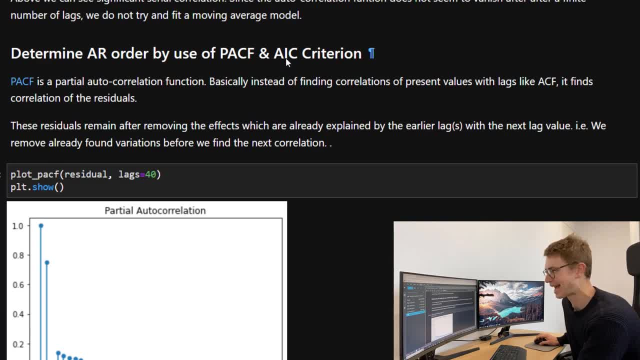 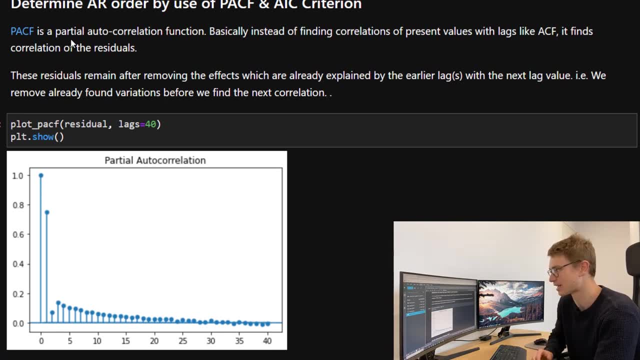 this by looking at the partial autocorrelation function and then the AIC criterion. so first off, the partial autocorrelation function. basically, instead of finding correlations are the present values of lags on all the data set from different days. it finds the correlation of the residuals. so what do? 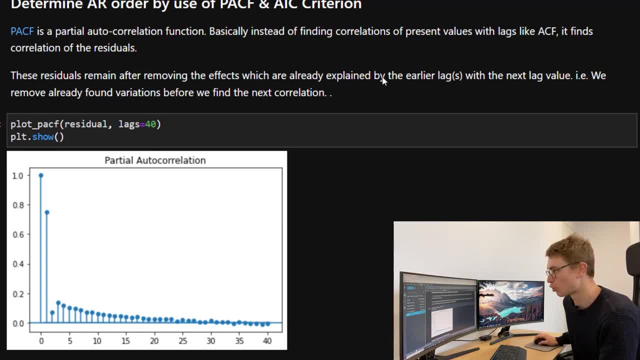 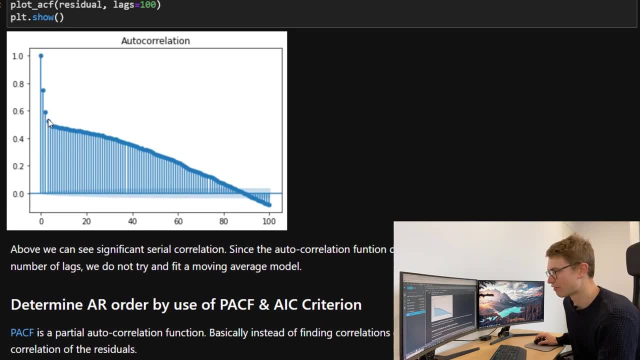 by that the residuals remain after removing the effect, which are already explained by earlier lags. so with respect to the next time lag. so here in the graph below we've already found huge explanation through the first two lags and that's not taken into consideration in the third lag. 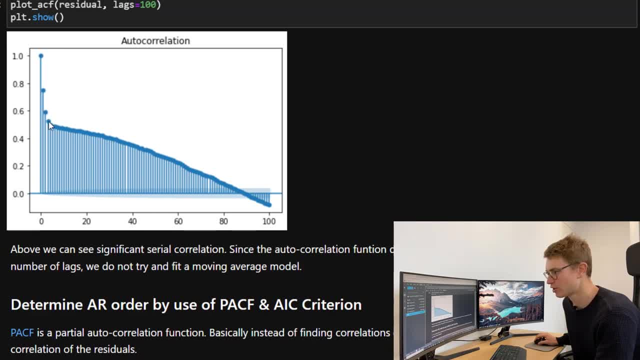 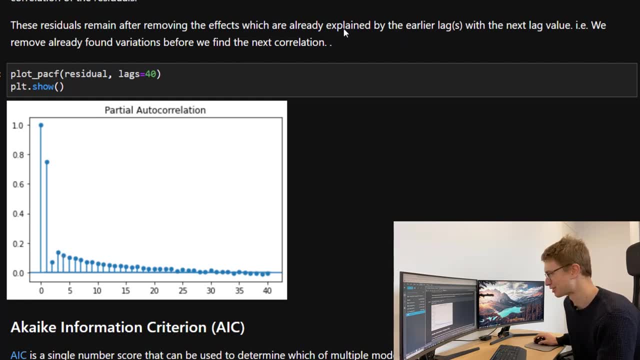 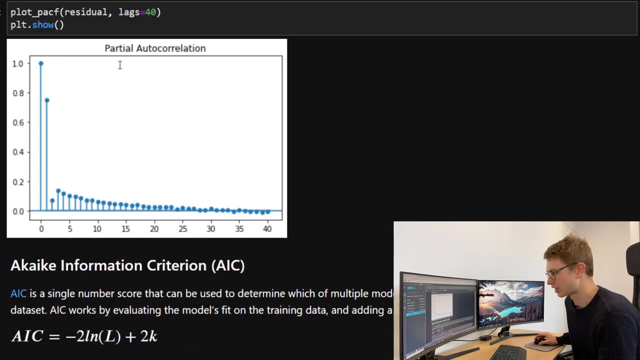 term there, whereas if you remove the effects of those first two then you get our partial autocorrelation on the third one in our partial acf function. so essentially we remove already found variation before we find the next correlation, and here we can see that there's a significant 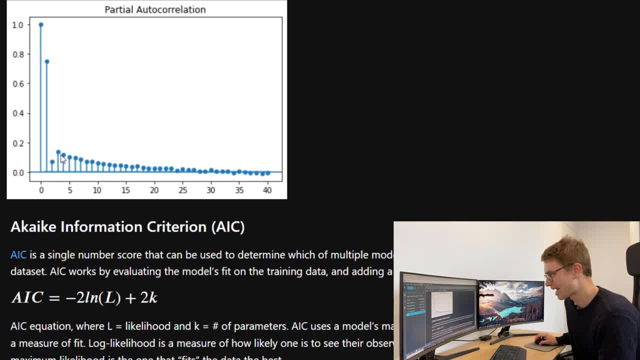 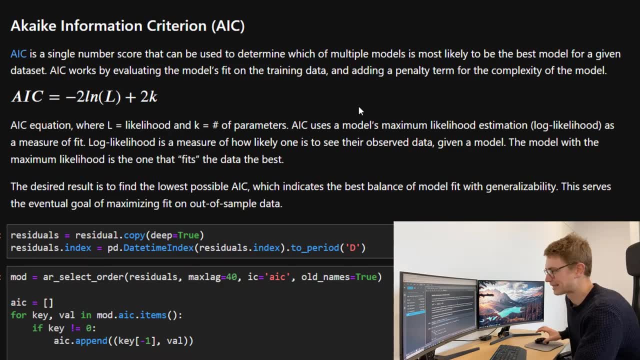 partial autocorrelation in our first two days, and then it kind of decreases all the way to 15 here, even 20.. now the archaic information criterion. so AIC, this is a single number score and essentially this is the number that we're going to be looking at in the next two days. 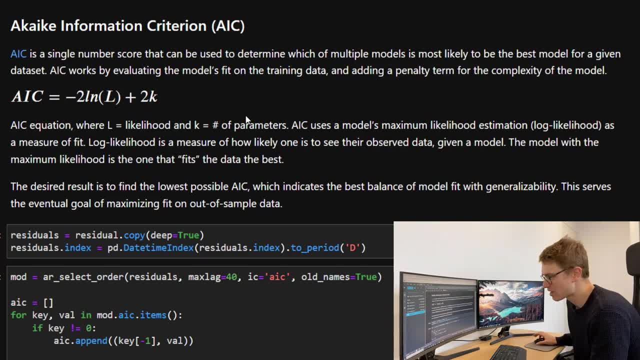 is just representative of model fit, and here we have two components. so this term here is about fit and this is using the log likelihood, and the likelihood is the maximum likelihood estimator of the fit of a particular model and k is just the number of parameters that that model has. so this 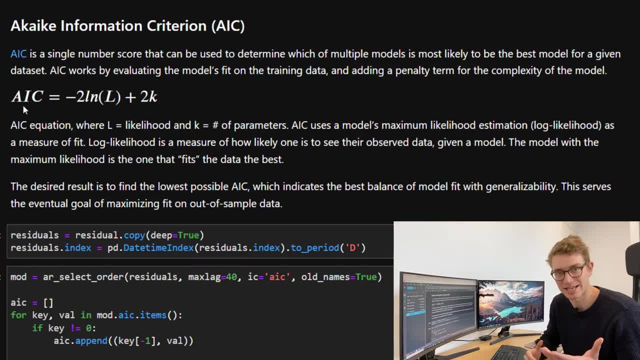 is about judging parsonomy. now, what we're trying to do here is get the best fit without over complicating or over numbering. so if we're overcomplicating, we have these two elements and we'll be fitting the model so as we increase the number of parameters, obviously the model 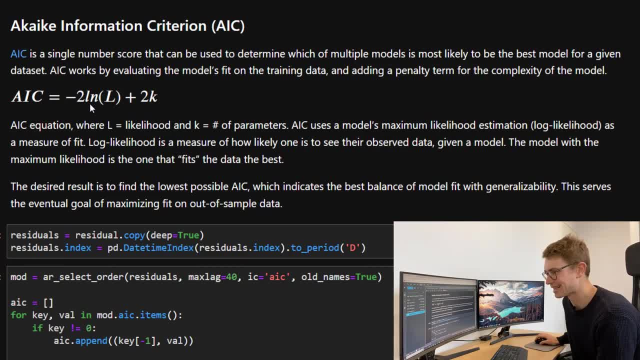 gets more complex. but we want to optimize and get the best fit. so the way that we're trying to optimize here we're using the AIC criterion to get the best fit. that it kind of reduces the number of parameters. so we actually want the lowest AIC value we can, but within reason so the best balance of model fit. 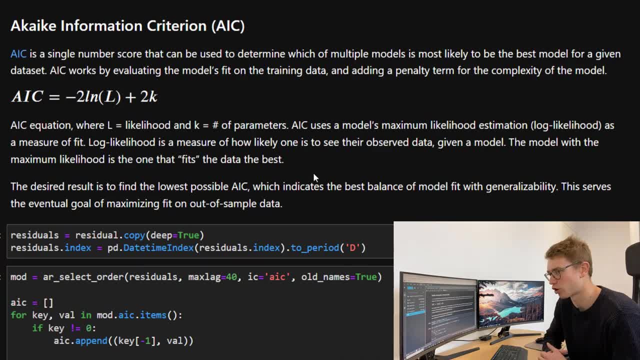 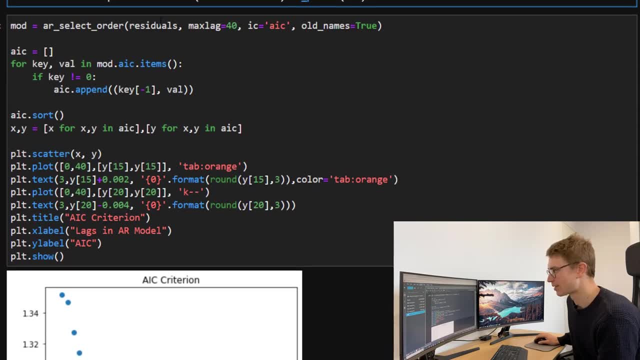 with generalizability. this is serving the eventual goal of actually maximizing our fit out of sample. so let's look at the residuals. we're going to test the residuals on a lag term up to 40 with our AR model and we're going to use the 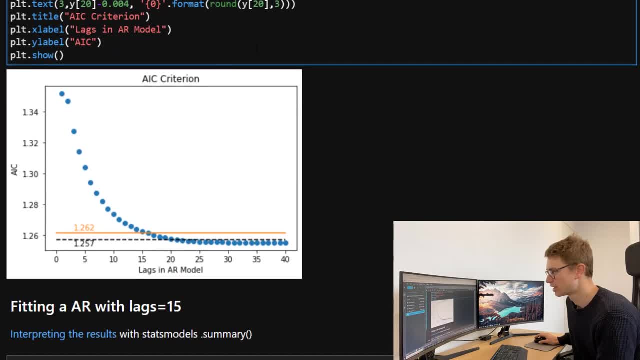 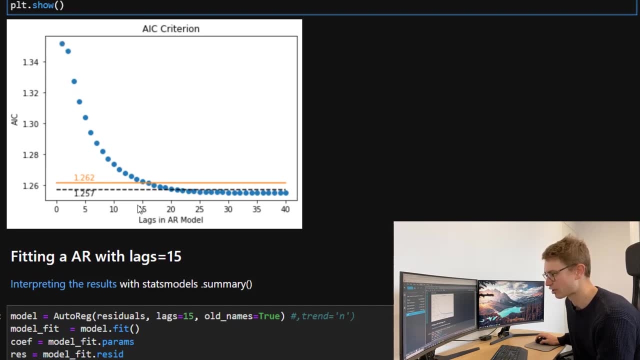 AIC model to actually sort on. so here in our graph we can see the AIC value that actually decreases as we increase the number of lags. that's included in our autoregressive model and, as you can see, as we get to 15 it goes down to about: 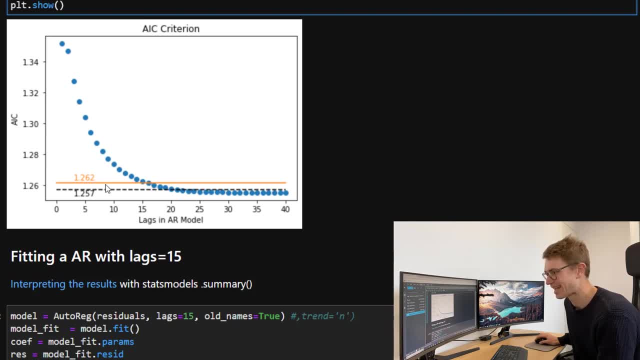 1.2- 6 and there's not really a huge decrease in the AIC after that. it goes down to 1.25 in our 20 and then even smaller decrease after we increase lag. so I'm going to make the decision here that we're going to fit an AR model with 15. 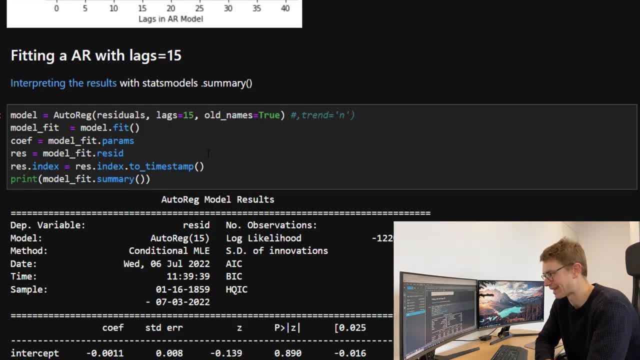 lags. now we're going to fit our autoregressive model with 15 lags and we're going to use the auto reg functions for that. on the residuals lags equals 15, and then we're going to fit the model. we can then look at the params. 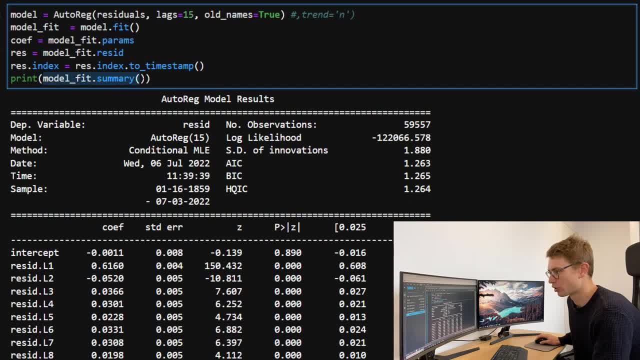 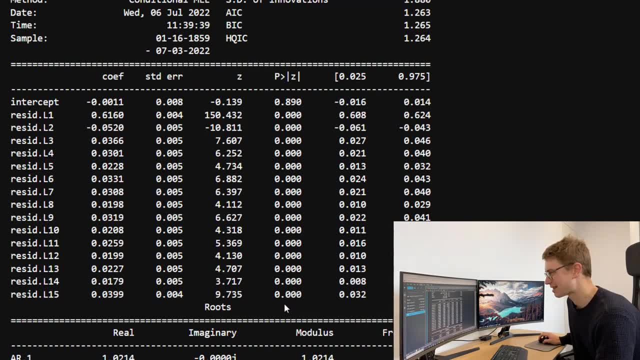 the residuals and we're going to, most importantly, look at the dot summary evaluation. so the most interesting road to look at is going to be our Z scores and then the probability of these Z scores. so, essentially, what we're doing here is the null hypothesis test. the null hypothesis test and being that, this 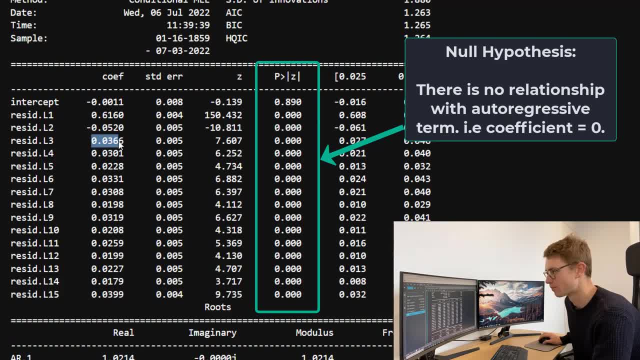 is equal to that, the coefficient is equal to zero. and what we wanted to do is we- if we, if that's really powerful and we have statistical evidence to prove that that is not the case, then we would reject the null hypothesis adding diff at a given critical level. so what we 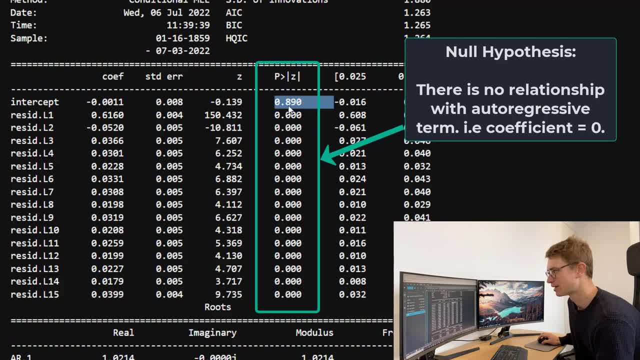 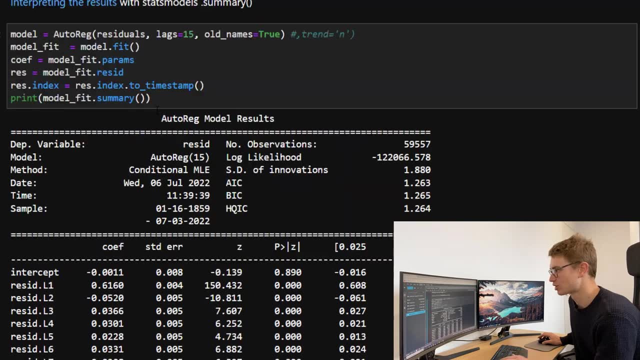 have here is that the intercept has a probability of 89. so if we set our critical value to, say, 5%, well then we cannot reject the null hypothesis that this is statistically insignificant. so what we're going to do is we're going to actually not going to include the intercept. so the way we do that is we 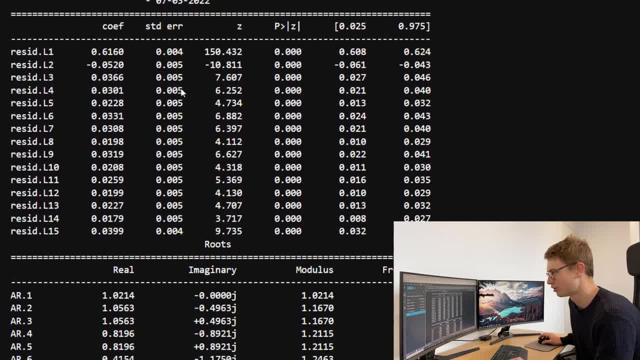 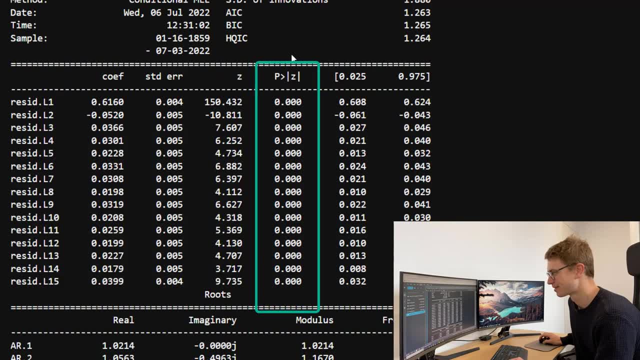 just include trend n for no, and essentially then we get our other coefficients without the intercept. now you'll see all the other, all the other p values here, for our estimates over these coefficients are zero. so we have to reject the null hypothesis and say that they are statistically significant and 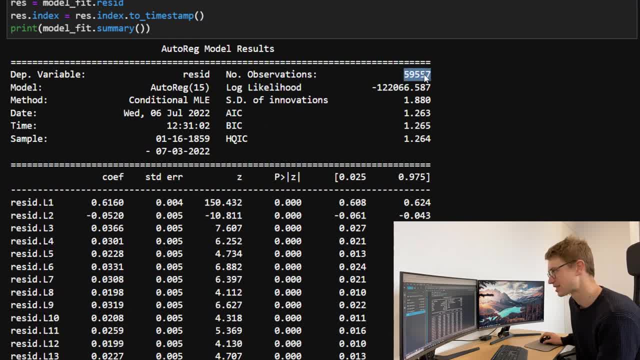 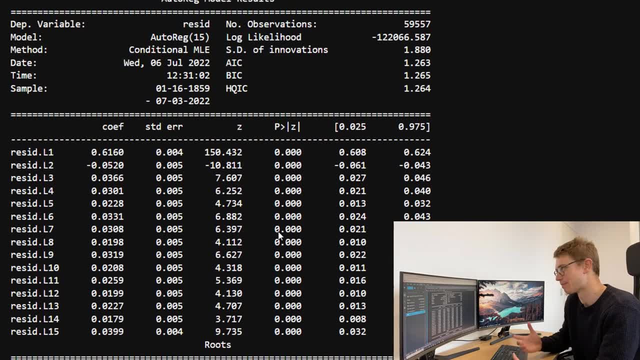 for such a large number of observations and given the fact that we need to capture this seasonality that is definitely present within the residuals, that makes a lot of sense to me. we also get the percentiles of this estimate, which are shown here. so our coefficient estimates are here, our parameters. that are estimates and then the percentiles. 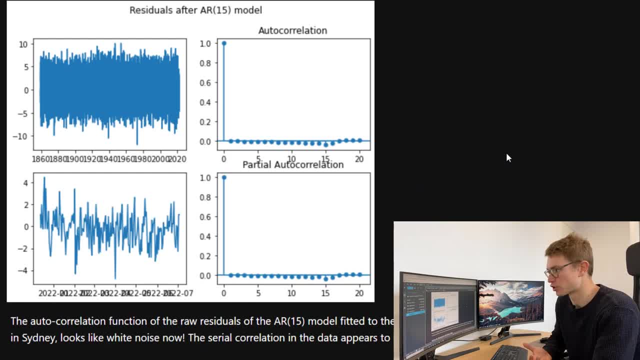 around. those estimates are here. so, taking a plot of what those residuals look like after we take into consideration that ar-15 model and we'll essentially now our residuals look like this, but we can't really see much there. so let's zoom in on the last 200 data points and you can see this. 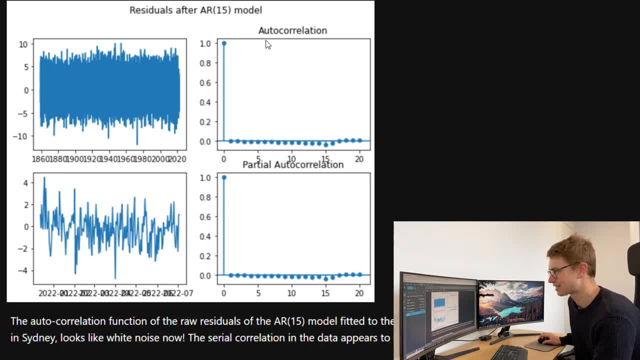 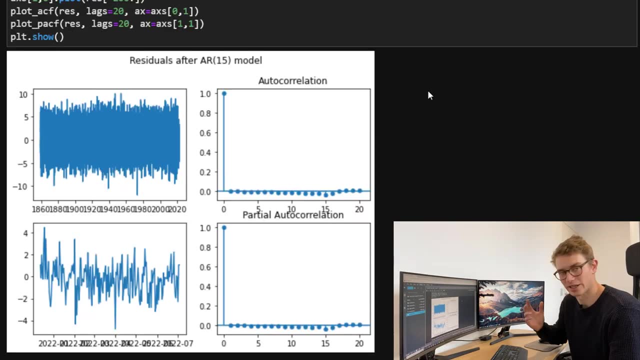 looks a lot more like a white noise process. essentially, now we have autocorrelation and partial autocorrelation functions that have almost zero autocorrelation between different lags, and this is exactly representative of a white noise process. obviously, there are other tests that you can do to 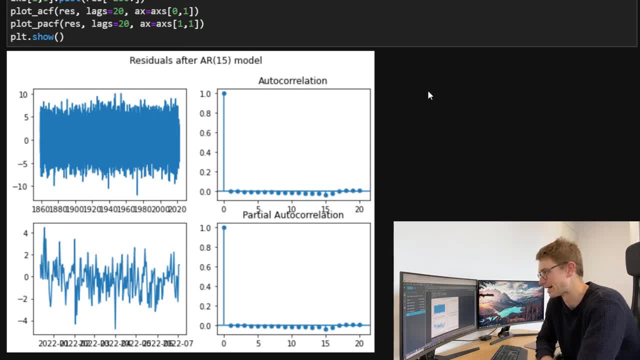 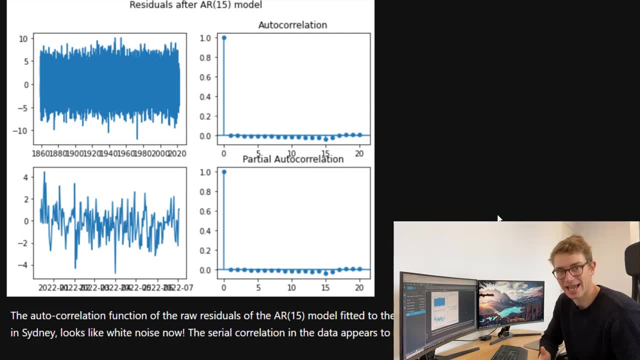 test whether it's a white noise process. we might go through that in another video. okay, so now that the serial correlation appears to have been captured within this AR model, now we have our trend component, we've got our seasonality component and then we've got a model for our residuals, which is an 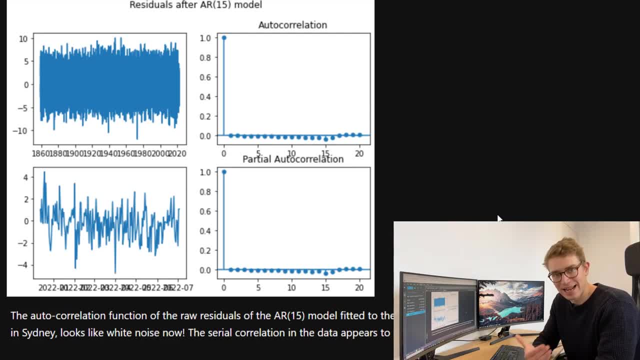 autoregressive model with 15 lag terms. so in the next video, instead of using classical decomposition, we're actually going to use Fourier series to represent our seasonal component of our data set. so see you in the next video. thanks for watching and I'll see you in the next one.